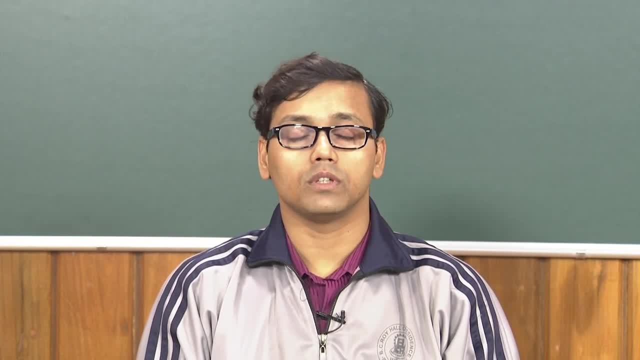 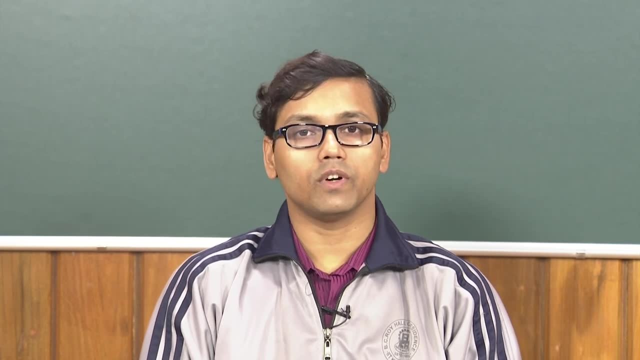 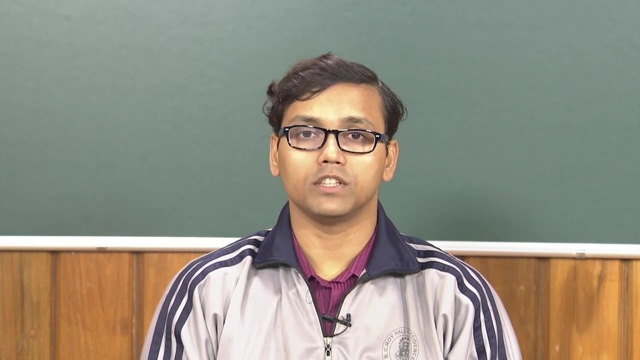 And that will be starting with this particular module in module 7, where we shall be talking about thermal reactors In previous 6 modules. if I would like to have a quick recap of that, in the first module you have learned about the very basics of nuclear energy production. 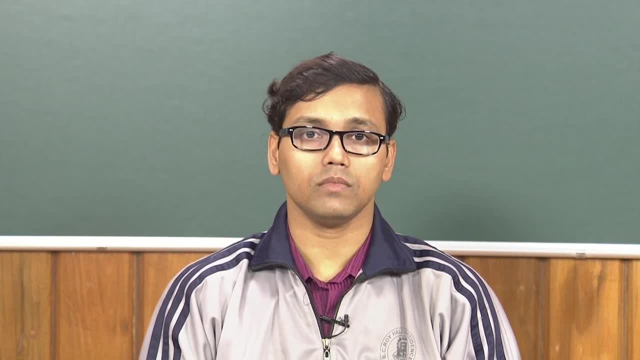 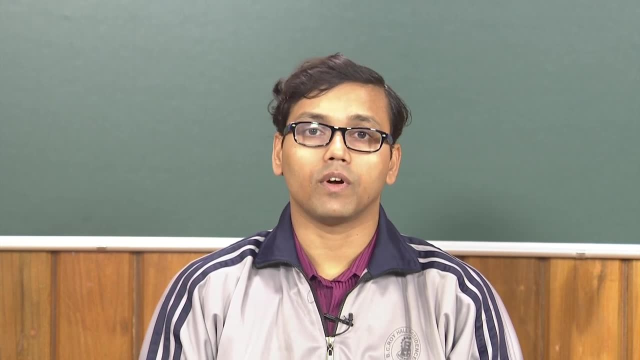 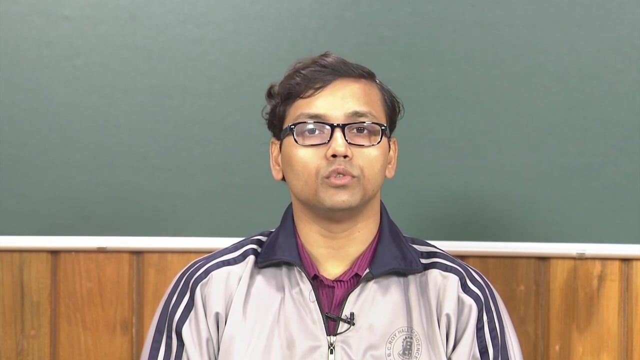 particularly through the concept of binding energy and mass defect. In the second module you are introduced to the topic of radioactivity, particularly in the topic of artificial radioactivity. you have learned that by striking the nucleus with a suitably charged particle we can induce radioactive decay in even in a stable isotope also, or stable nucleus. 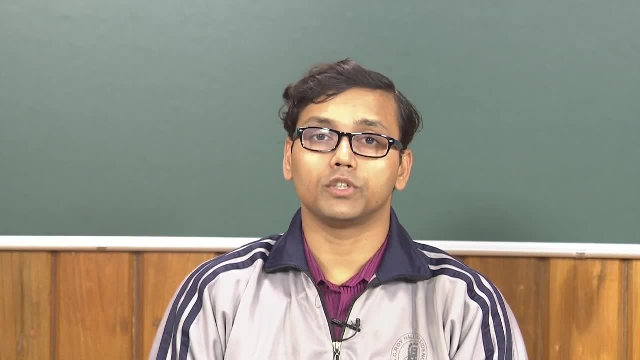 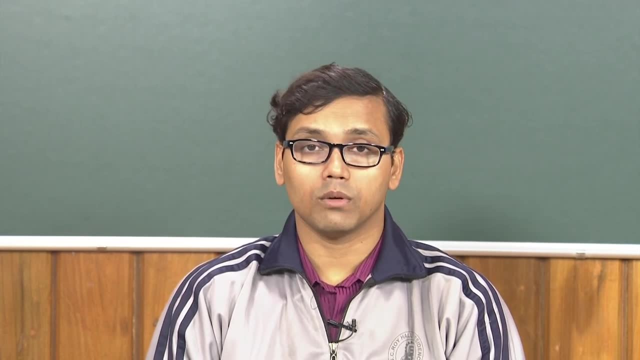 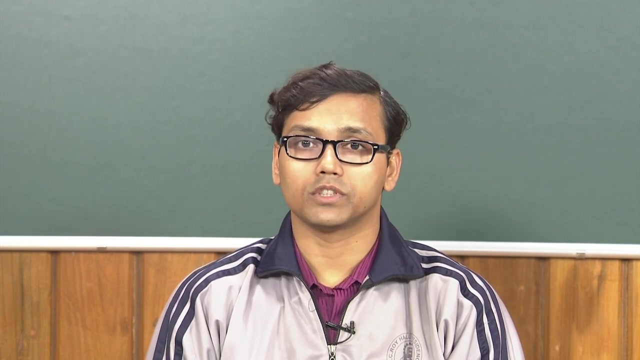 But the nature of such nucleus, or I should say the outcome of such an interaction between a neutron and nucleus. that will depend upon both the energy level of the neutron and also the nature of the nucleus, And from there we got the concept of nuclear cross section. 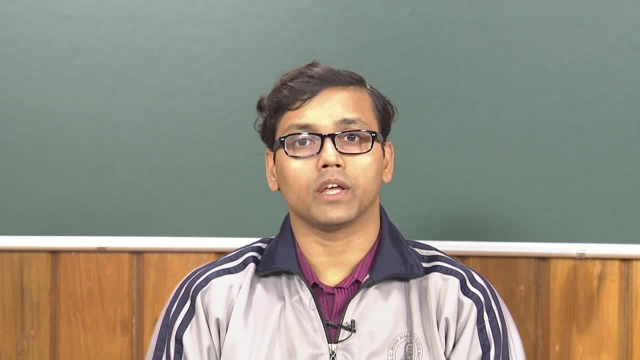 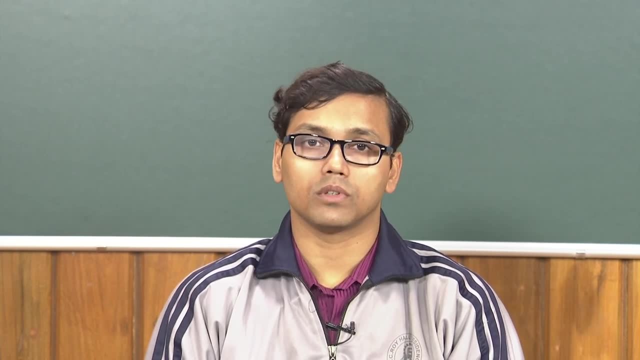 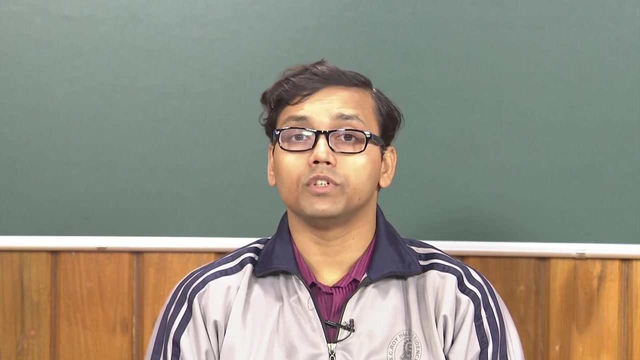 Only a few. certain nucleus can have fission cross section of any significance And in the third module we have discussed about those isotopes or those nucleus and also more detailed about fission. In the fourth module we talked about the neutron flux profile because generally 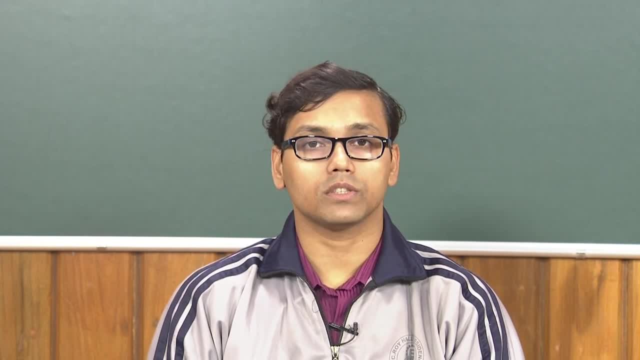 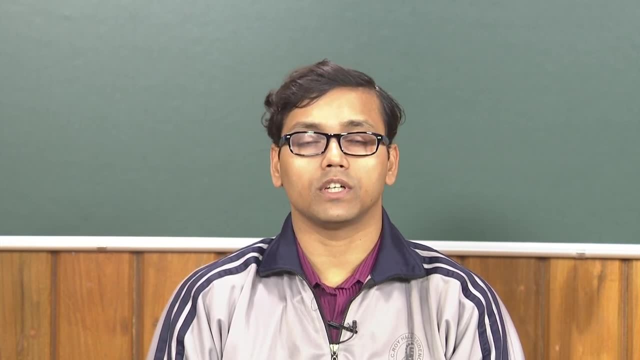 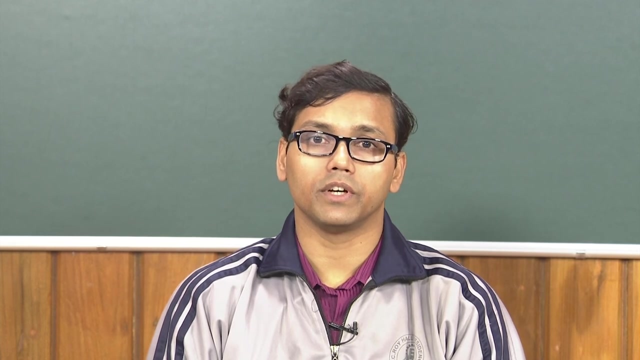 the energy released during fission reaction is directly proportional to the neutron flux And therefore we have discussed about the profile of neutron flux that we can get in different kinds of idealized reactors in order to sustain a critical reaction, or I should say in a in a critical reactor. what should? 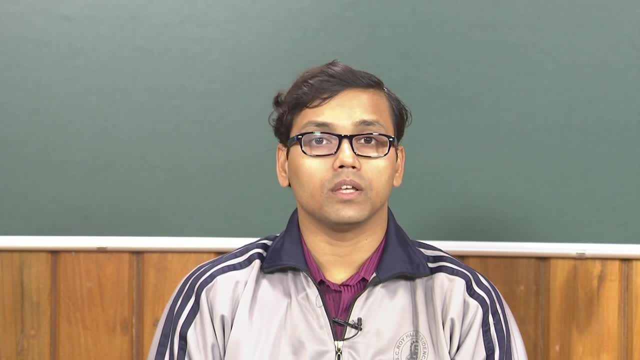 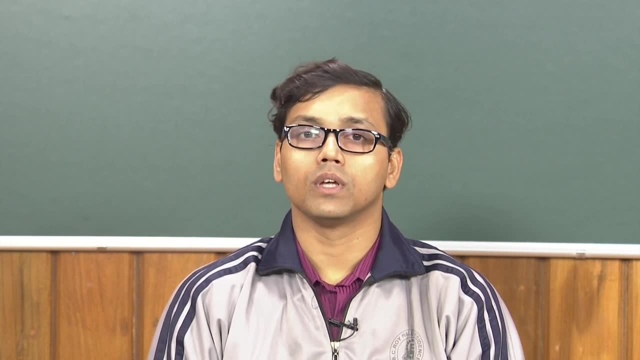 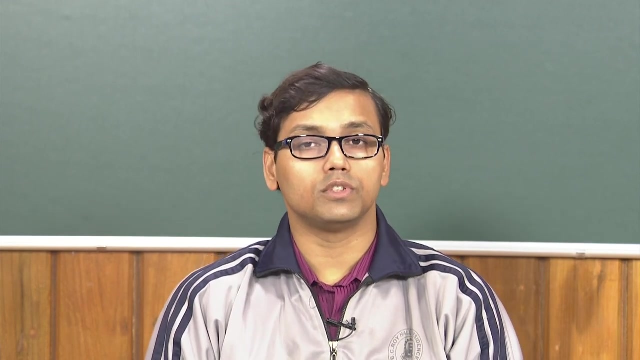 be the neutron flux profile that we have seen there In the module number 5. we actually came out of the reactor a bit, or I should say came out of the ah neutron interaction part where we discussed about the thermal hydraulics, That is, the energy which is produced. 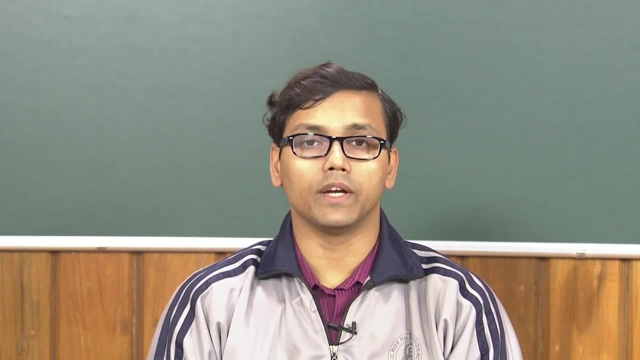 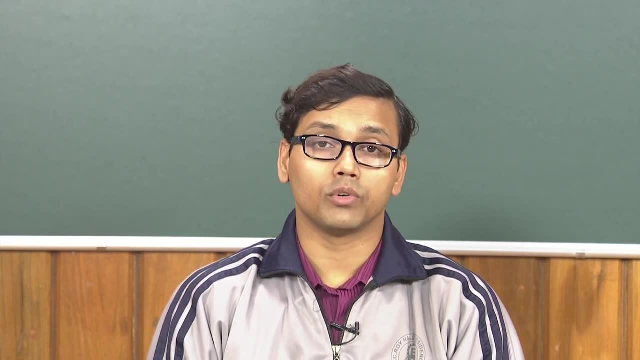 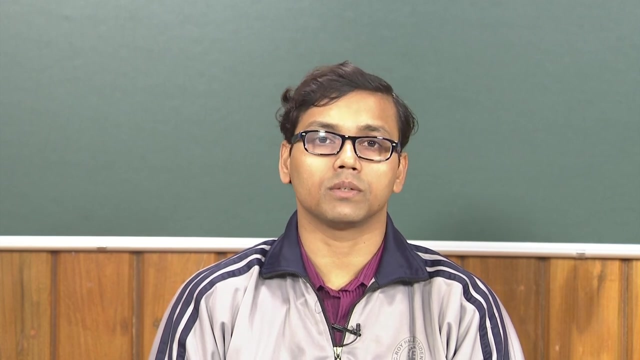 during the fission reaction that can get transferred to the coolant. that we have learned in the fifth module. In the sixth module we again discussed about the control issues, particularly in a transient operation, because some planned transients or some unplanned transients: how to control? 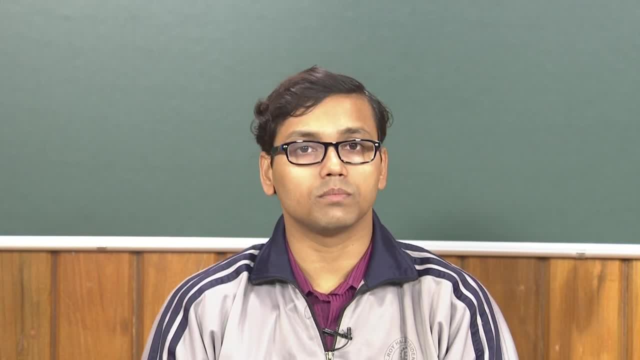 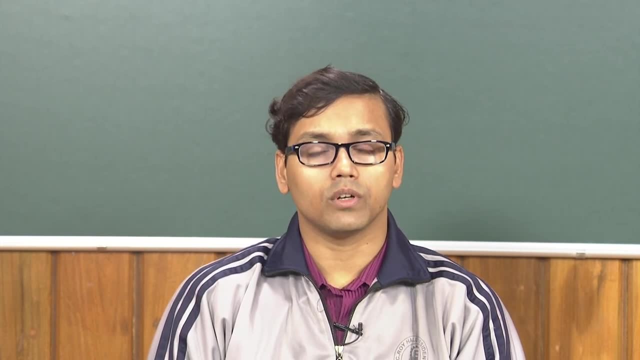 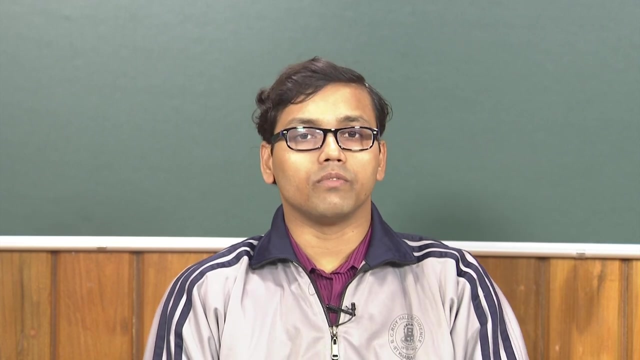 that that kind of issues that we have discussed in the sixth module, where you have learned the terms like important component of nuclear reactors, such as the control rods, chemical shims, etc. And also we have discussed about the role of various parameters, such as the delayed 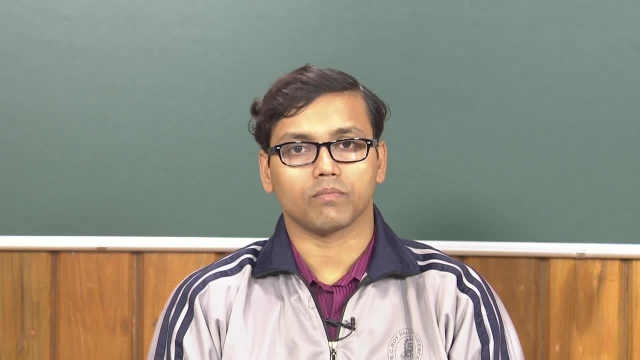 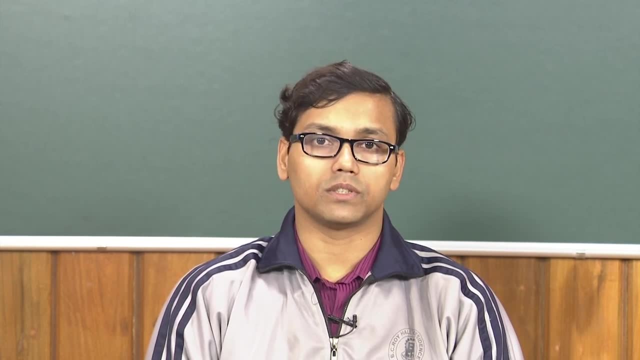 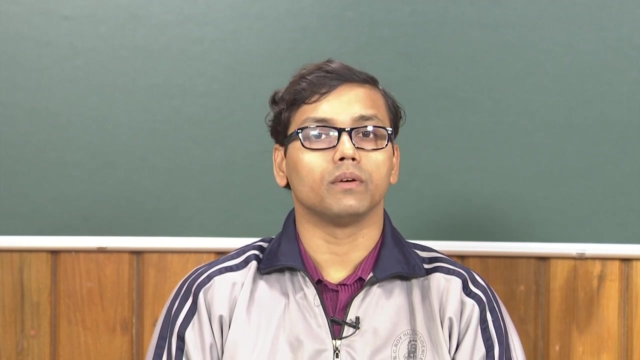 neutrons, fuel, burn up temperature, etc. So now we know that in any reactor generally, we have four different substances. Number one is a fuel. A fuel is the one which goes through the fission reactor. Fission reaction thereby produces large amount of energy by virtue of its own radioactive. 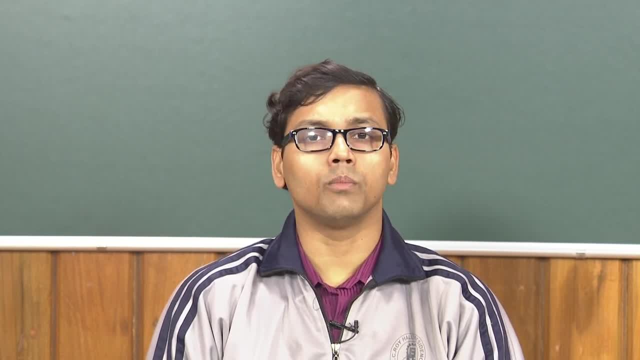 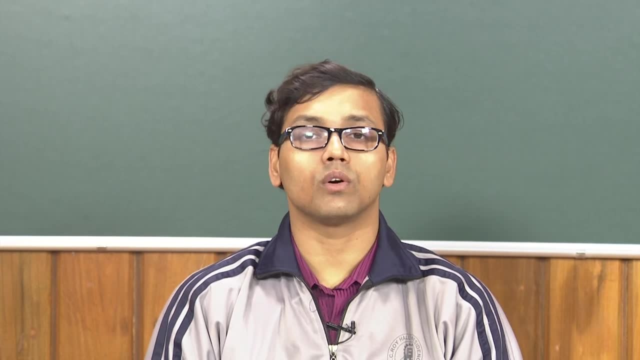 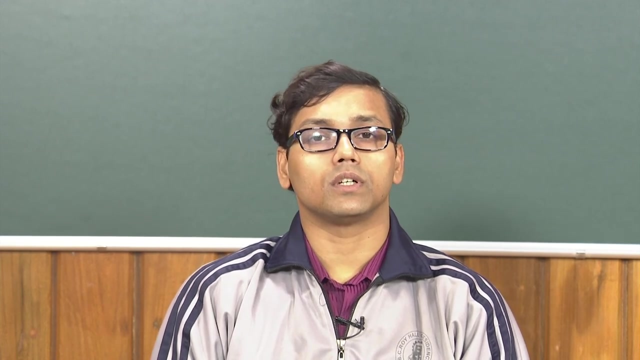 decay or nuclear decomposition. Commonly, uranium-235 nucleus is the fuel that is used, but uranium-233 or plutonium-239 can also be used as fuel. Second substance is moderator. Moderator is the one which which allows the neutron to go through multiple scattering. 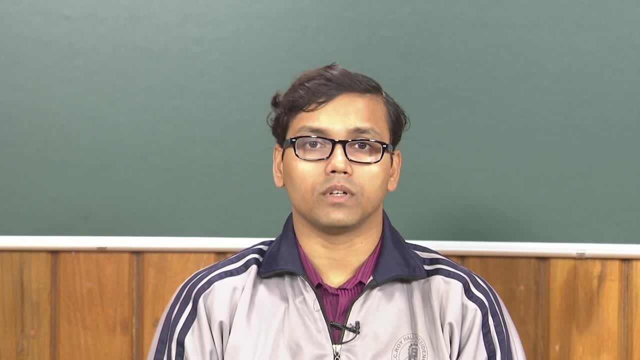 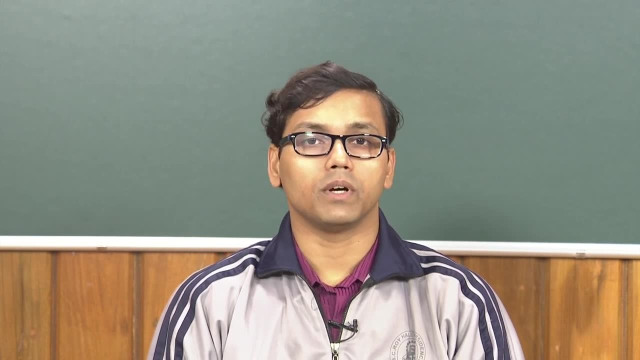 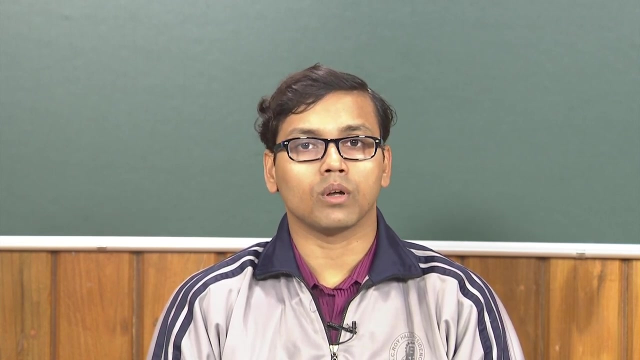 thereby converting The prompt neutrons to the thermal neutron level or high energy fast neutrons released from a fission reaction gets converted to the thermal neutron level by repeated scattering or repeated collision with the moderator nucleus, And that is very important because the conventional fuels like uranium-235 or plutonium-239 has. 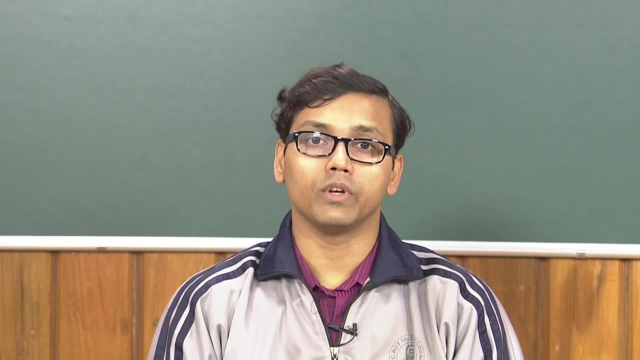 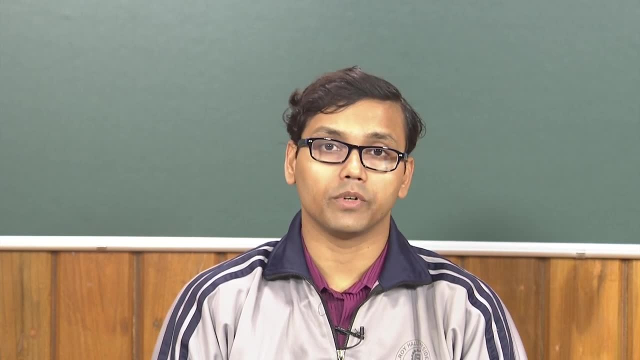 much higher neutron fission cross section when they are subjected to thermal neutrons. That is why moderator has plays a very important role in increasing the power of the neutron. So we have discussed about this, Thank you. So we have discussed about the performance of the reactor. 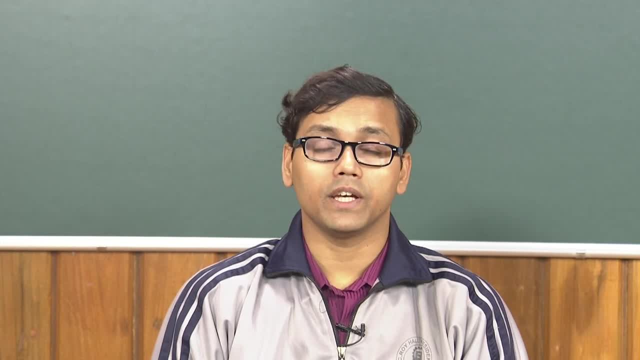 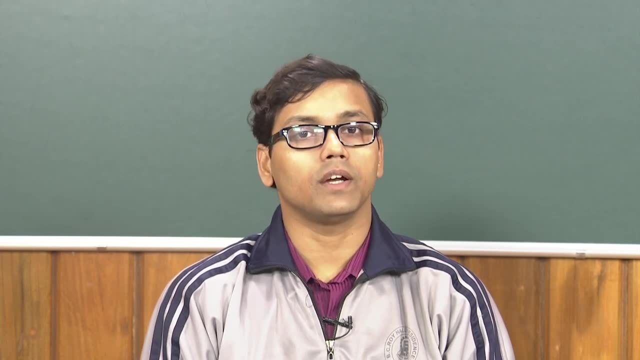 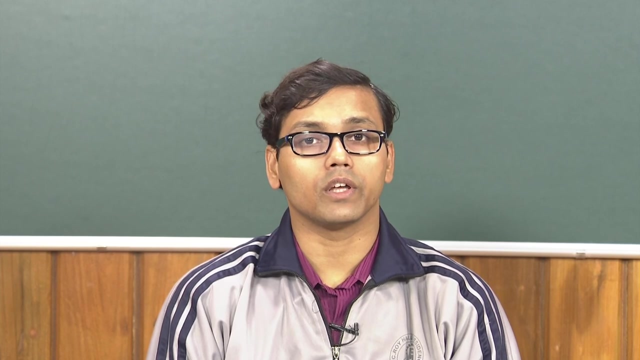 So we have discussed about the performance of the reactor. The third substance is coolant. The energy which is released by fission that needs to be transferred to the coolant, which actually will be interacting with the external world, and the net output from the reactor generally be manifested in the form of energy rise or energy gained by the coolant itself. 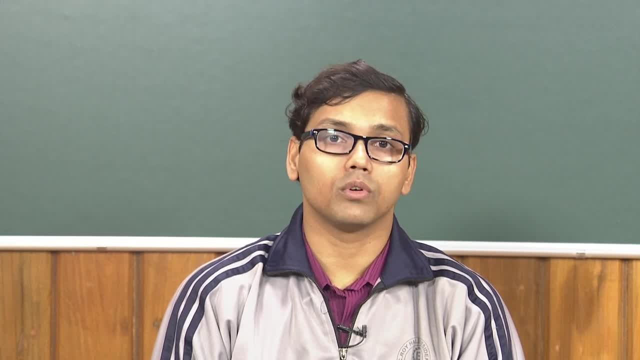 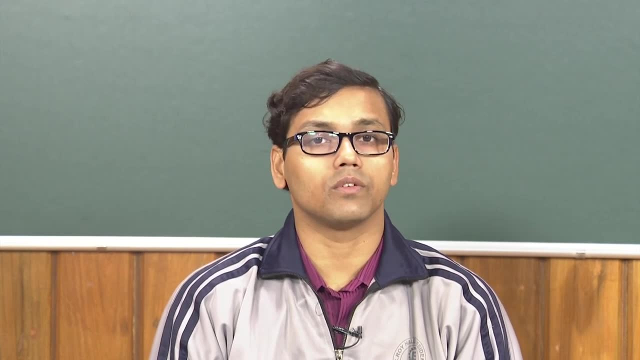 And number 4,. just, we have studied in the previous module the control rods or control electric equipments. Control rods are universally present in any kind of reactor. Certain other reactors we have also discussed about this. reactors can also have chemical shim or burnable absorbers, but they generally all use similar. 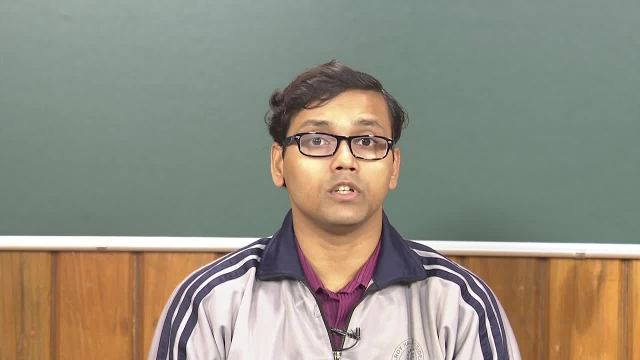 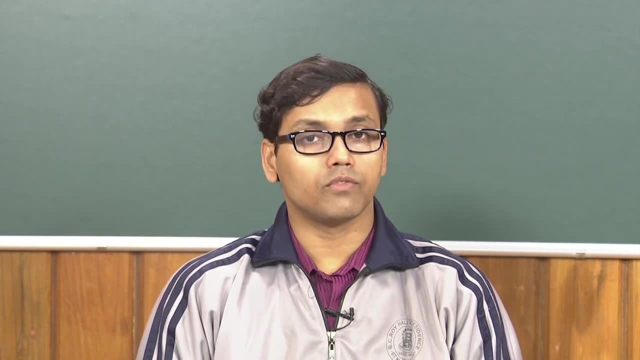 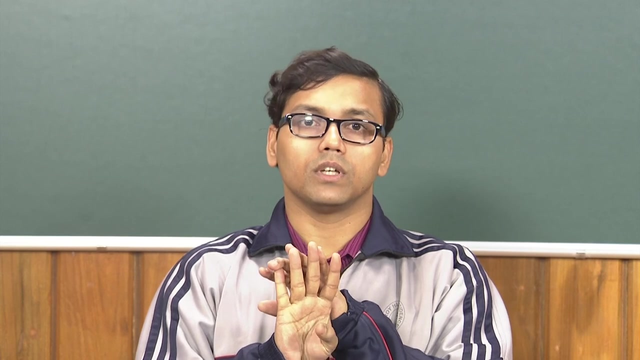 kind of materials like boron or cadmium or hafnium or gadronium which has very high neutron absorbing cross sections. So we generally commonly can have four types of elements, that is, fuel, moderator, coolant and also the control equipments And we can 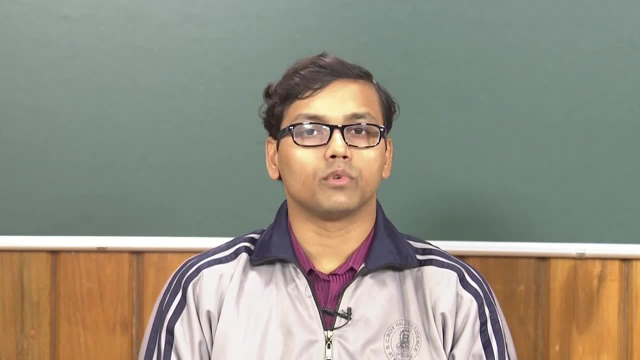 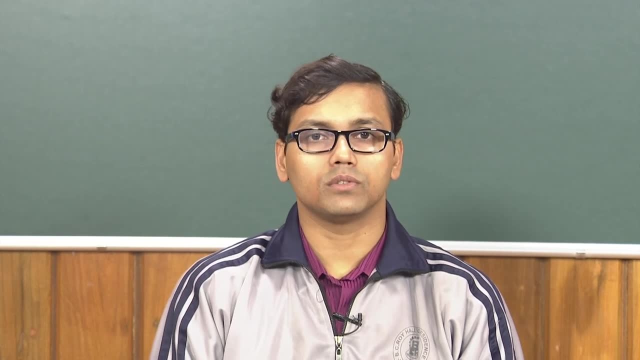 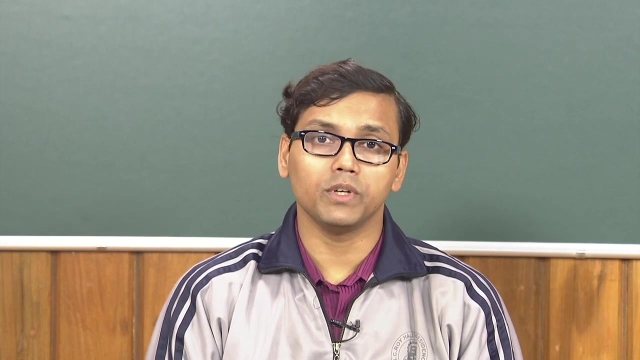 also have certain things like the fission products, the neutron poisons, etcetera, that are generally only a byproduct of the fission reaction, So do not need to be considered at the moment, But the four that we have mentioned, depending upon their combination and also 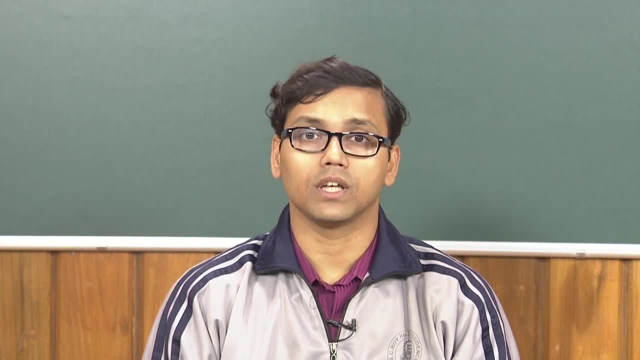 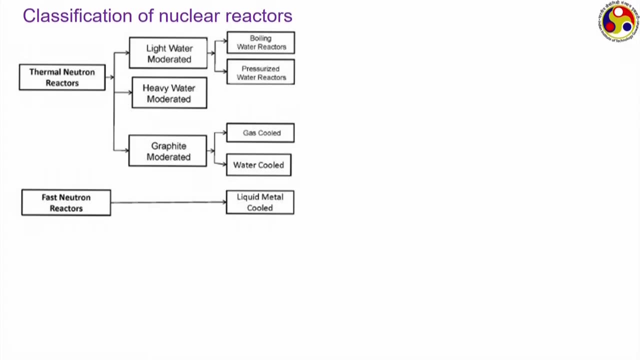 their orientation. we can have different kinds of reactors, and that is precisely what we are going to discuss in this lecture Now. nuclear reactors can we can use- this is the initial point of contact. Now how be broadly be classified into 2 categories depending upon what kind of neutrons they? 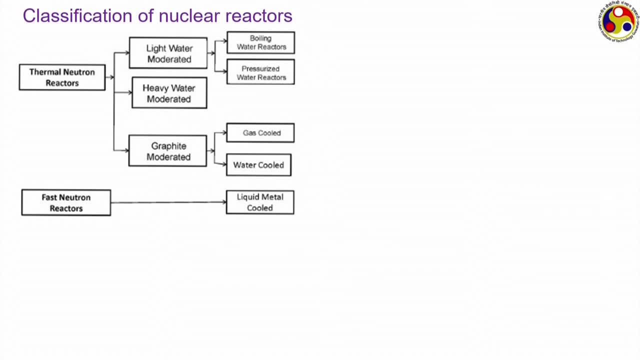 use. When they use fast neutrons, we call them fast neutron reactors. when they use thermal neutrons, we call them thermal neutron reactors, And thermal neutron reactors are the most common one. more than 90 percent of the reactors may be more than 95 percent of the reactors. 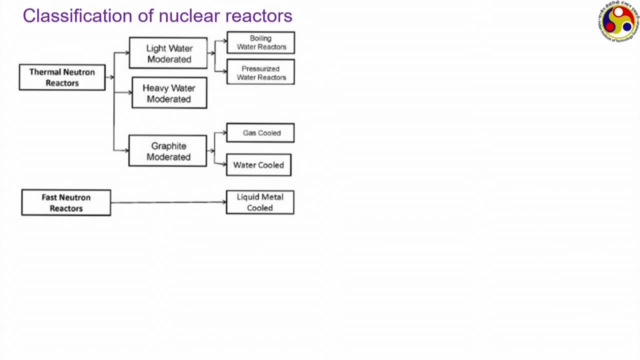 which are available commercially throughout the world are actually thermal neutron reactors. because of certain reasons which we shall be discussing later on, Thermal neutron reactors again can be classified depending upon what kind of moderator they are using, Like ah 3 principle kind of moderators which are used in thermal neutron reactors. 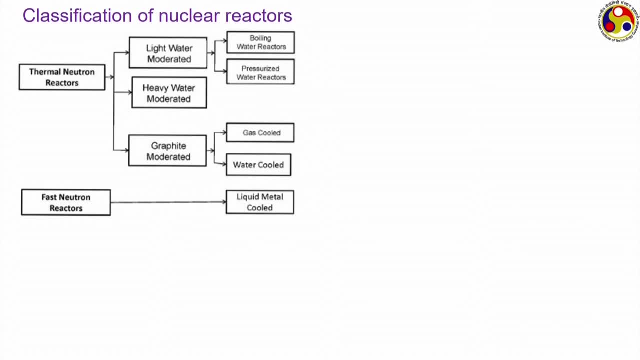 are common water, heavy water and also graphite. Here in the slide, the term light water is mentioned. I probably have mentioned earlier also that the term light water is ah, frequently used in the nuclear field. However, it is not a proper term because this is just the ordinary water that you are. 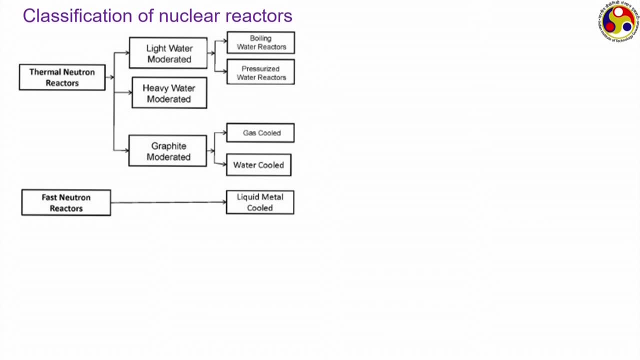 talking about. There is, of course, heavy water, but there is nothing called light water. Still, this, being such a common terminology, is the nuclear field. we have to keep on using this. ok, So we can have. ah, depending upon moderator, we can have 3 types of thermal neutron reactors: the ordinary water reactor or the light water. 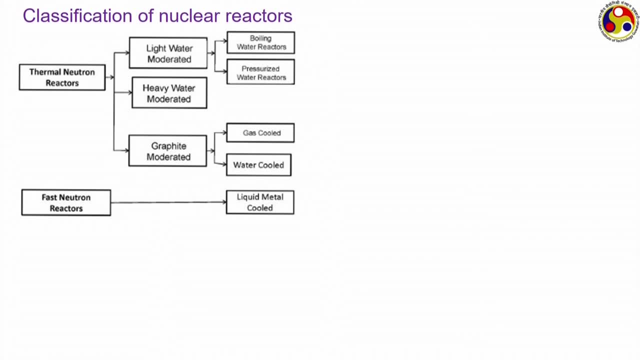 reactor, heavy water reactor which uses D 2 O as the moderator and, of course, the graphite moderator reactor. So these are the 3 types of thermonuclear reactors. So we can have 3 types of thermonuclear reactors. 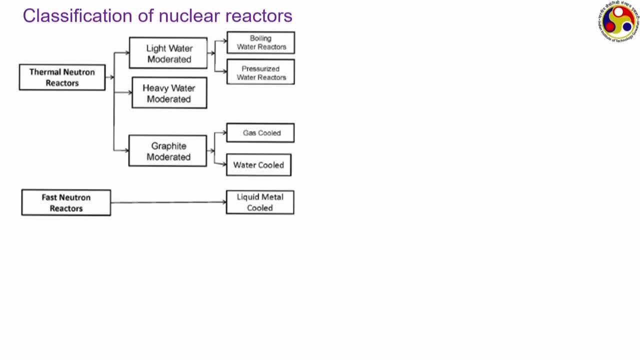 And the light water moderator reactor again can be classified into 2 categories depending upon the physical state of the coolant that they use. It can be pressurized water reactor where the coolant remains under single phase because of high system pressure or the coolant can undergo ah can undergo a phase change. then we call that a boiling water reactor. 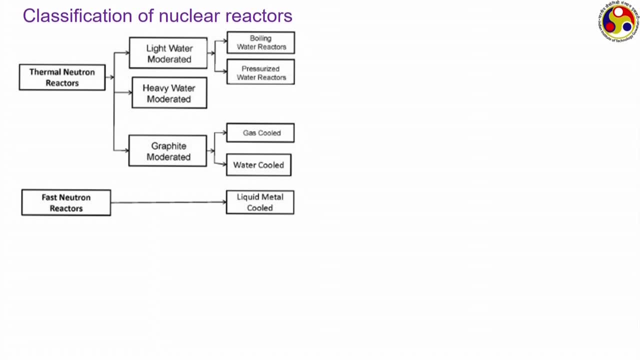 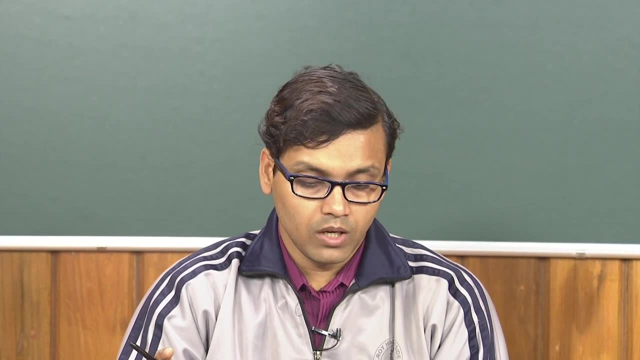 The graphite moderator reactor again can be of 2 types: One which uses some kind of gas-like carbon dioxide or helium as the coolant, other which uses water as the coolant, The fast neutron reactors. ah, by definition it needs to use the fast neutron, So there. 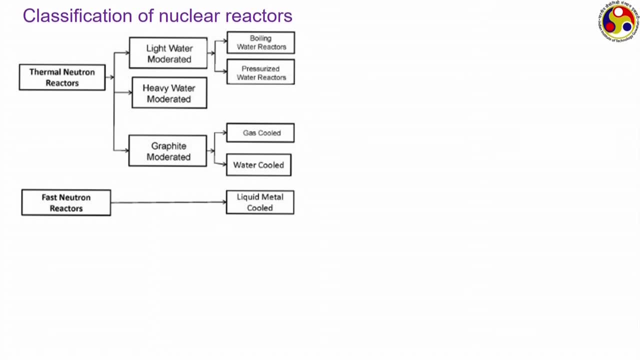 is no moderator there and it generally uses liquid metal as the coolant. This is a typical ah, neutron, ah flask profile and ah for the thermal neutrons reactor. the thermal neutron reactor generally operates in this zone Where the neutron energy is of the level of 0.025 electron volt, whereas the fast neutron reactors operate mostly in this particular 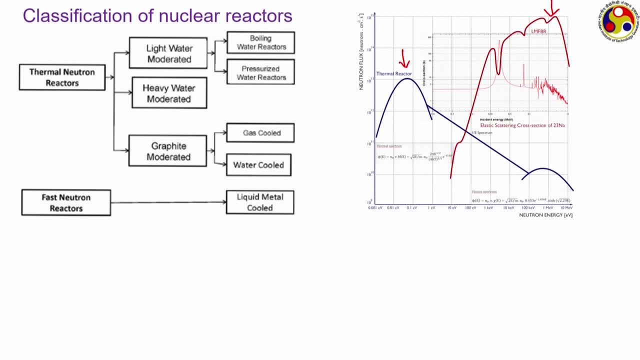 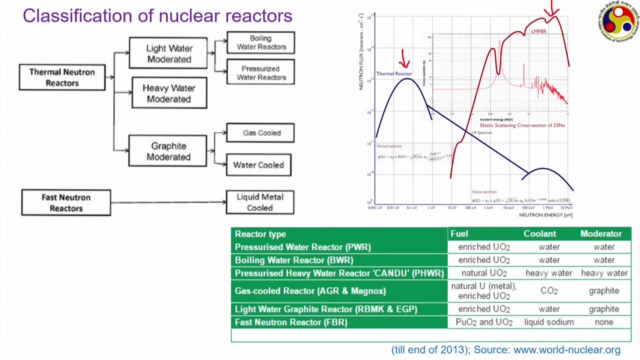 zone where the neutron energy is very high, of the level of 1 mm v or can be even higher. These are the most common or conventional nuclear reactors that we can find throughout the world, The, and, as mentioned here, we can have generally 5, 6 types. I should say ah, pressurized. 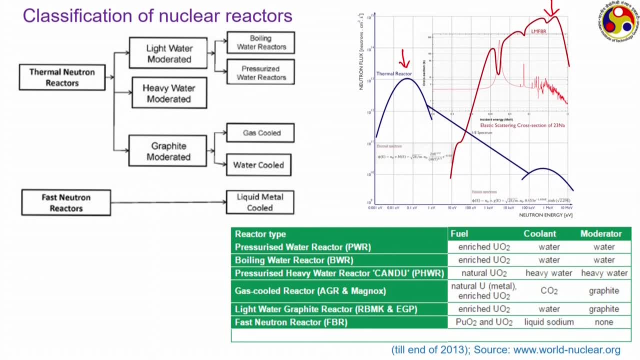 water reactor, or PWR, boiling water reactor, or BWR, then pressurized heavy water reactor reactor, gassed cooled reactor, light water graphite reactor and also the fast neutron reactors. Out of this- ah, all this 5, they are actually thermal neutron reactors, because they use thermal neutrons for to induce the fission. 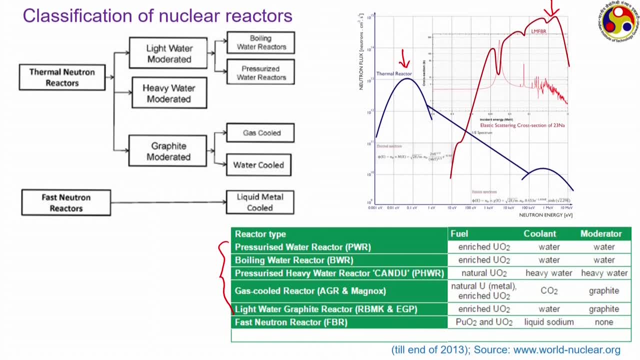 reaction, but the last one. there is a fast neutron reactor that uses fast neutrons for the ah to induce the reaction And we can also see in ah the first 2, that is, PWR and BWR. Water acts as boron. 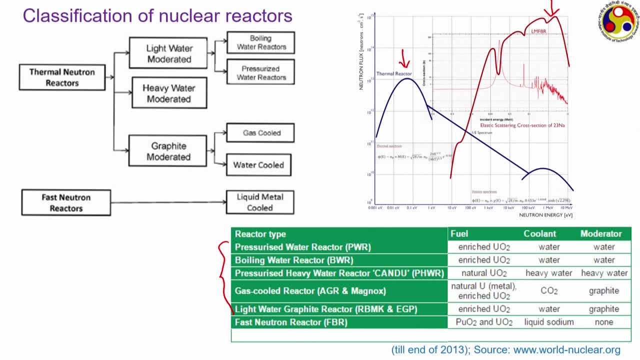 Both moderator and coolant. whereas in case of pressurized heavy water reactor, heavy water is used as both moderator and coolant, In case of gas cooled reactor the moderator is graphite and coolant is a gaseous material like carbon dioxide and, in light water, graphite. 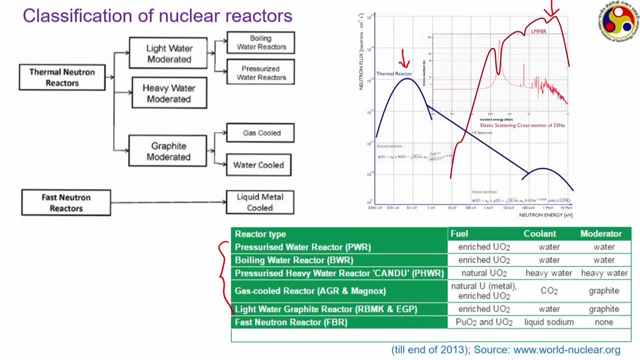 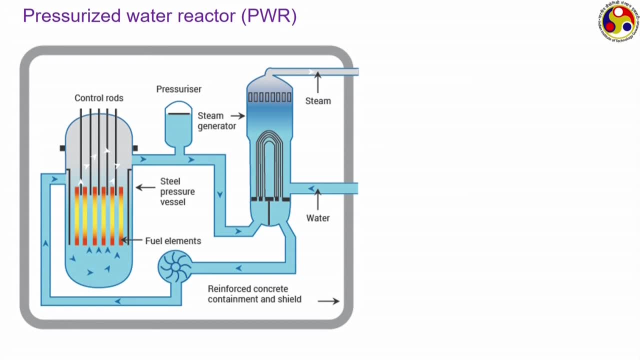 reactor. the coolant is water, but the moderator remains graphite. Now the first one, probably the most common one, that is, a pressurized water reactor, or PWR. Pressurized water reactor is the most common type of nuclear reactor that you can find throughout the world, in different countries, like in United States, United States in several 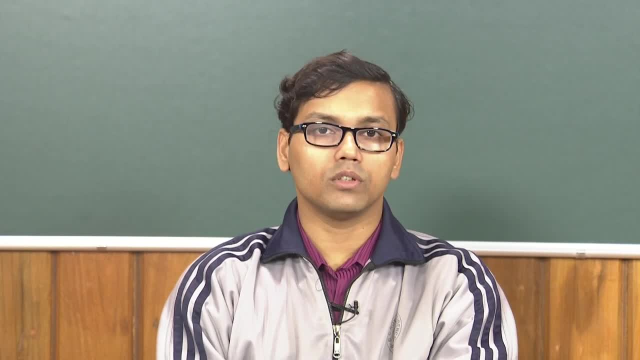 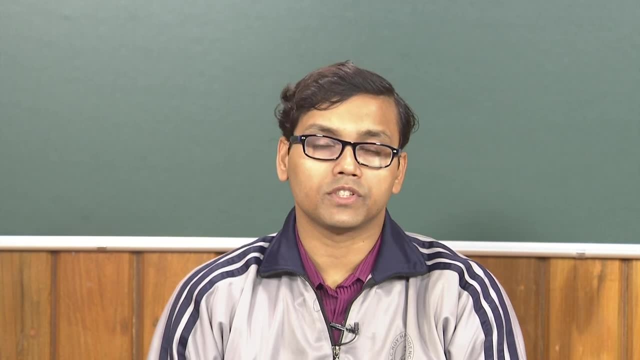 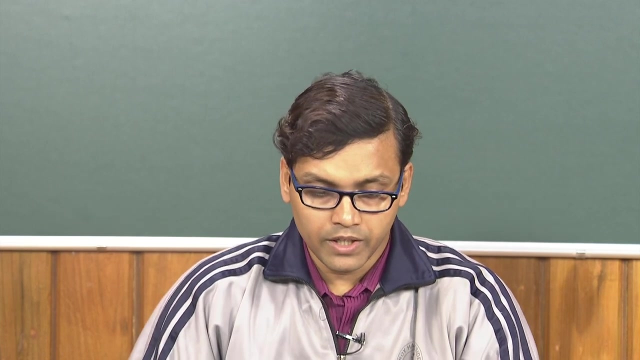 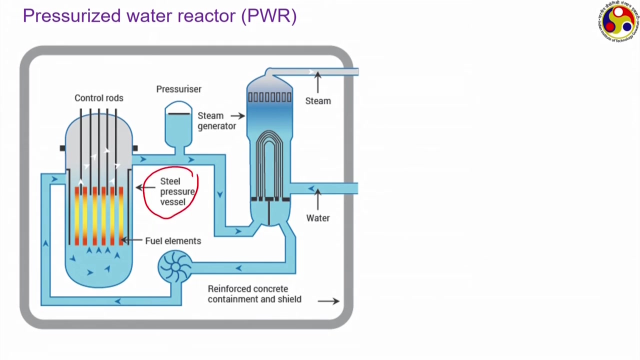 European countries like Germany or France, and also in several other parts of the world. Actually, in India, the first nuclear plant that was established at Tarabor, Maharashtra, that reactors are also of PWR category. In case of a pressurized water reactor, the main component is a pressure vessel. This pressure vessel, generally made of steel, is the one 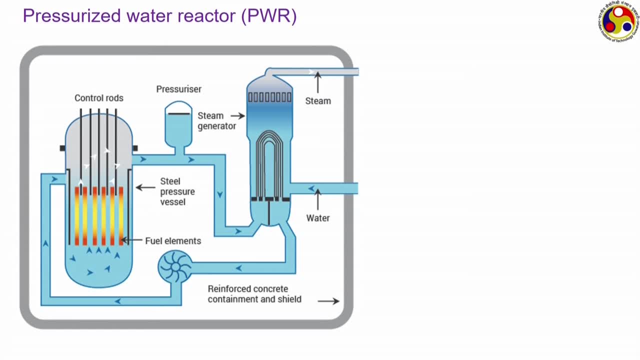 inside which all the fission reaction happens. Inside the pressure vessels we may have the fuel elements, ah, which can be of the shape of cylindrical rods or maybe rectangular pallets. They are placed following certain kind of orientation and control rods. the control rod material is generally boron. 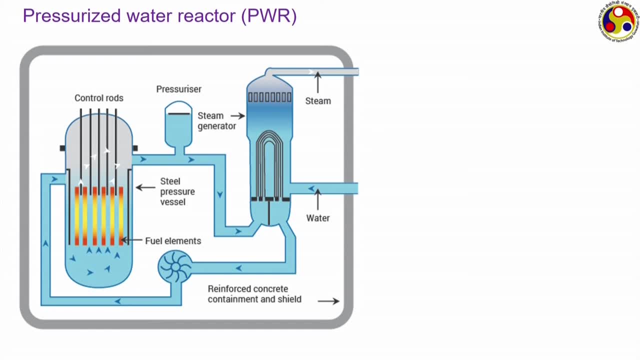 Or some compound of boron, like boron carbide or boron oxide, which are allowed to pass through the gap between these fuel elements So that they can capture some certain portion of neutrons available there, depending upon their level of insertion. It was mentioned in the previous. 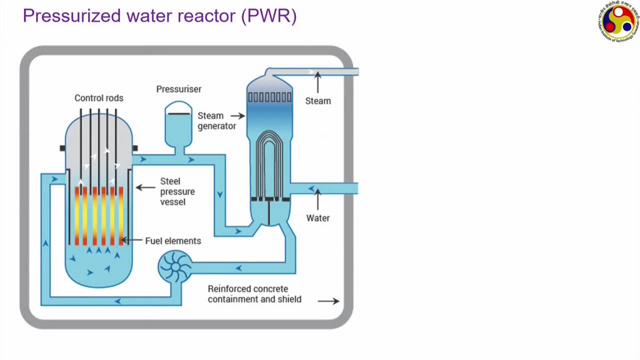 lecture- also a previous module- that in PWR the control rods are inserted from the top and hence the control rod connecting mechanism. So this is the control rod which is used for driving mechanism, particularly the spider that is mounted at the top of this pressure vessel And this fuel elements and also the 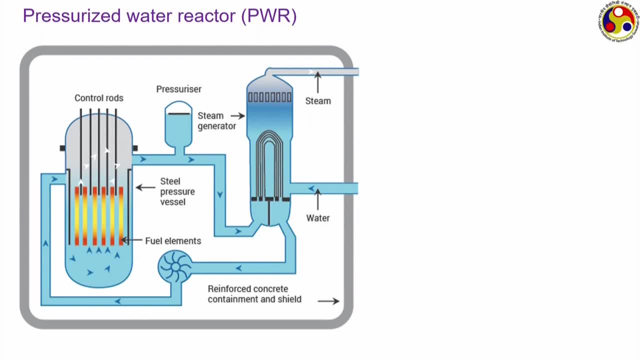 control rod. they are completely immersed into the moderator, And the moderator in this case is water that is only liquid water. No phase change is allowed in pressurized water reactor and the water that is as coolant and moderator that we are using, that must remain as single. 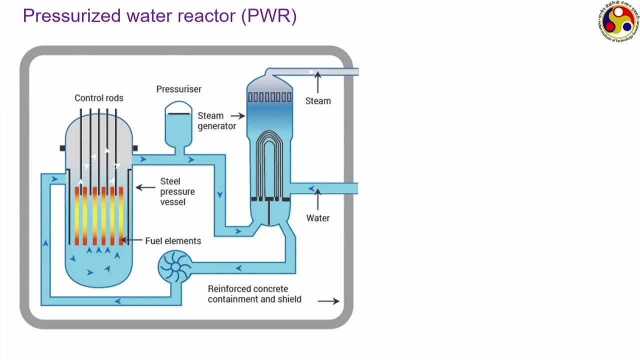 phase liquid And it is a relatively pressurized water reactor, The. So, if we follow the diagram, the liquid- generally cold water- that enters the reactor through a channel like this- Inside the channel, it passes through this line and then is allowed to move upwards through the fuel or bit through. 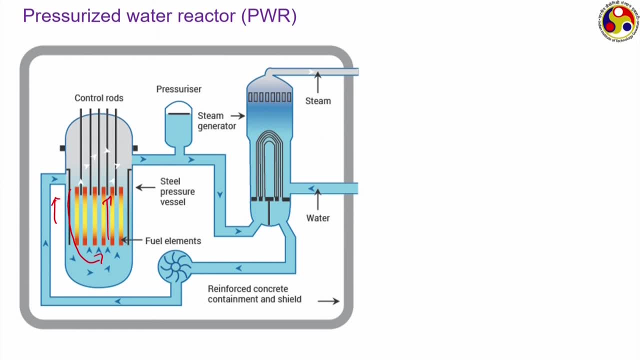 the spacing between two neighbouring fuel rods or fuel pins And therefore it is able to capture the energy that is released by the fusion of the neighbouring ah fuel, partamo d verticals or fuel isotopes. So when it comes out of this fuel bundle, then this same water. 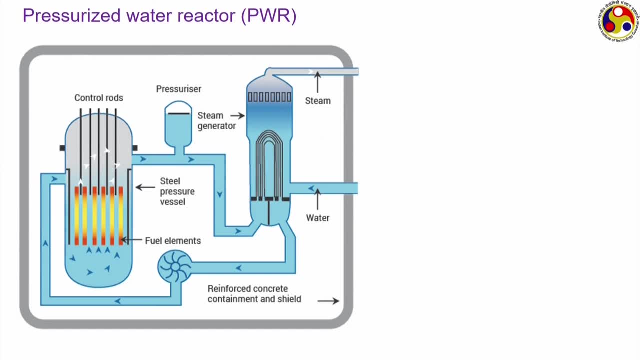 is at a reasonably high energy level and if we can maintain the water under liquid condition, then definitely its temperature will be much higher than the inlet temperature. The water comes out of the reactor here, and so between this point ah, which we can mark as 1, which is the inlet for this water, and this is the 2, which is the outlet of the water, 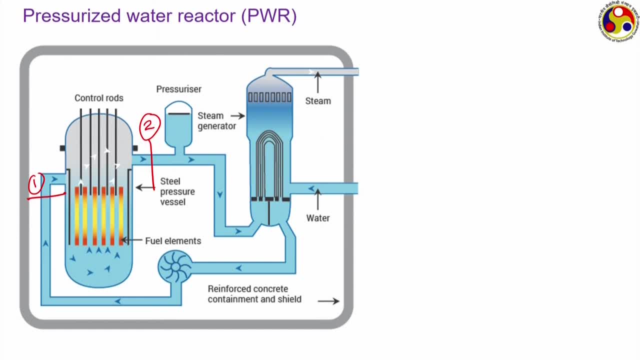 between these 2 points there will be significant difference in the energy level or enthalpy of this water, but physically both of them will remain as liquid. Now, the component which ensures this liquid status is this pressurizer. We shall be talking about pressurizer afterwards. 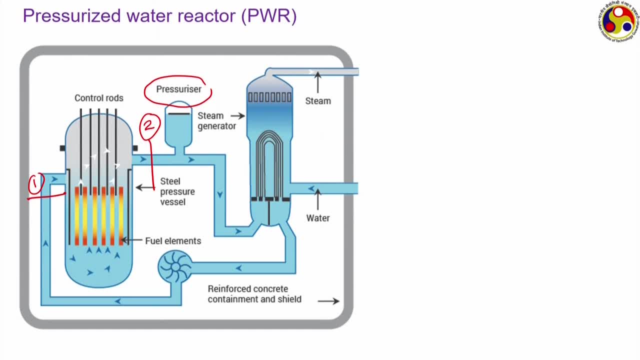 but this liquid water then is allowed to come to a steam generator inside the steam. this liquid water- high temperature liquid water, I should say- travels through a heat exchanging water. So this liquid water then is allowed to come to a steam generator inside the steam. this liquid water- high temperature liquid water, I should say- travels through a heat exchanging. 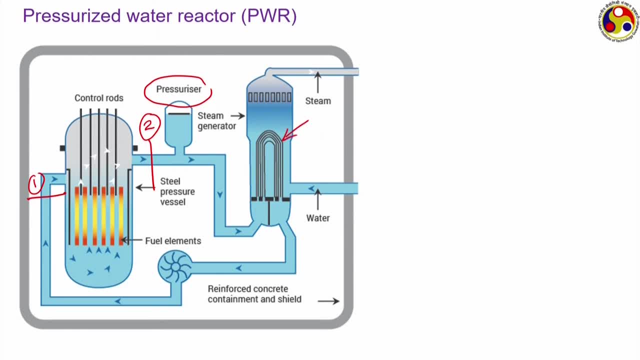 pins or a heat exchanging areas. outside of that, again, water is flowing, but that water is not allowed to mixed with the water that is coming from the reactor itself. rather, the water coming from the reactor is at a high energy level or high temperature, and therefore 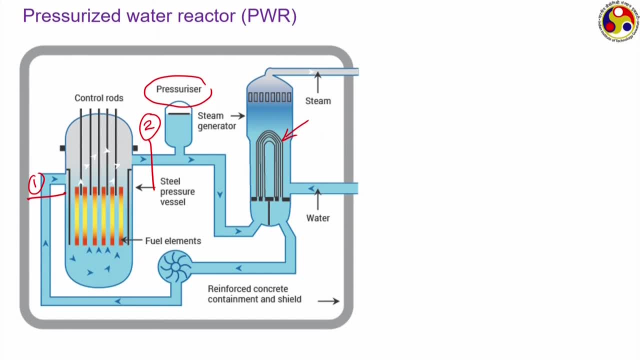 it is able to transfer the energy to the water which is outside, which actually is the coolant, and then this water from goes back to the reactor. Therefore, we can clearly say that in case of pressurized water reactor, we are using water as the moderator, as the coolant, and also as the working fluid, The steam, which 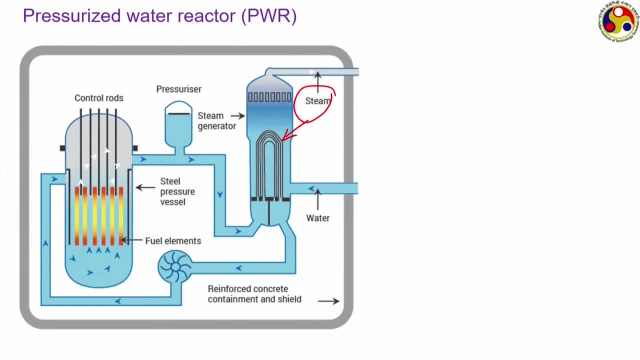 is produced in this steam generator, this one that is allowed to go through a turbine where it will give you the work output. So the moderator and the coolant, and also this water in the outside circuit, all are water from chemical point of view, but the 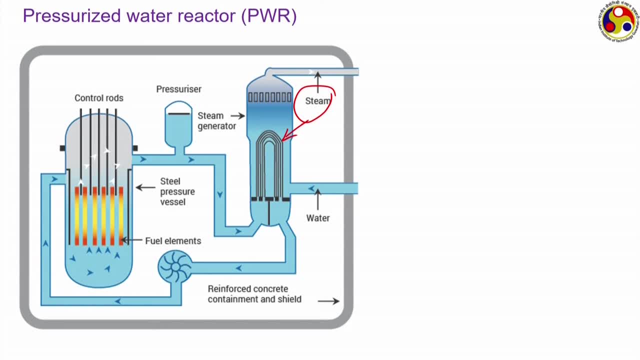 water which is used as the moderator inside the reactor, that is, that is not the working medium. rather, the working medium will be water, but some other body of water or some separate quantity of water which is circulates only in the external circuit. So a pressurized water reactor employs water as moderator, coolant and also working fluid. 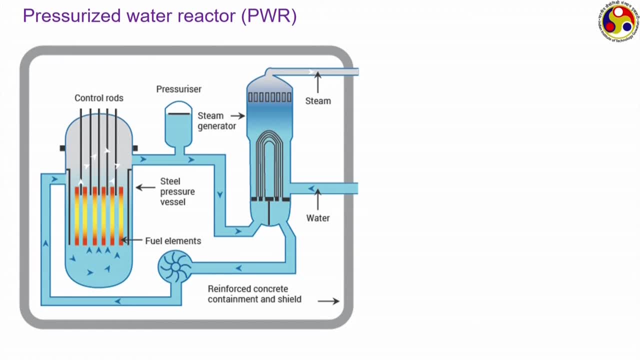 So the water is not a working substance, but the working fluid remains separated from the moderator. Now, in order to maintain this liquid status, we have to maintain a very high pressure, and pressurized water reactor operates at a high pressure level of something like. 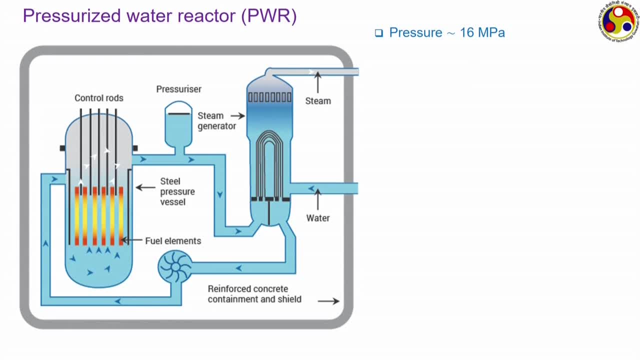 15 or 16 mega Pascal- that term pressure also comes from there- or pressurized, I should say. Now, at such high pressure level of 16 MPa, the saturation temperature- water will also be very high, which is somewhere around 340 to 350 degree Celsius. 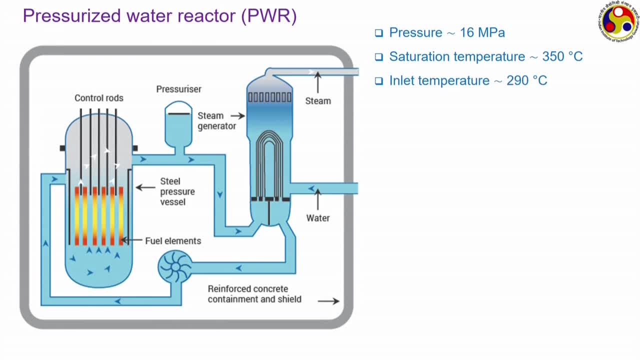 Now the water which is which is entering this reactor core. it is at this particular point this water temperature is something like 290 degree Celsius, And then the flow rate of this water is controlled such that at the exit the temperature is limited something to 320 to 325 degree Celsius, which is well below the saturation temperature of 350 degree. 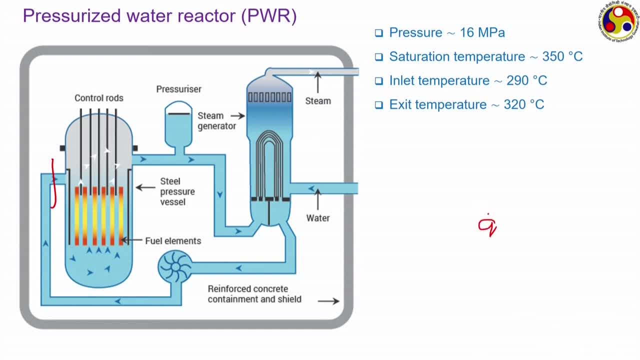 Celsius. Now if we have some idea about the energy produced in the reactor, that is, q dot, then we can always write an energy balance equation as m dot c, So c p into T 2 minus T 1, where m dot is the mass flow rate of this water coolant c. 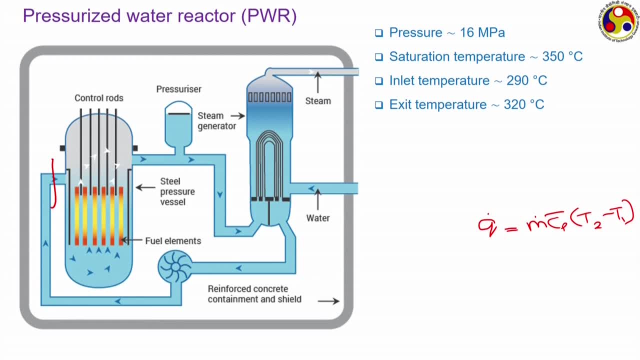 p bar is the average specific heat and T 2 is the outlet temperature at this point, whereas T 1 is at this particular point. So if we have some idea about this q dot and c p being generally a known quantity, then you can control the m dot by a pump which is mounted here. 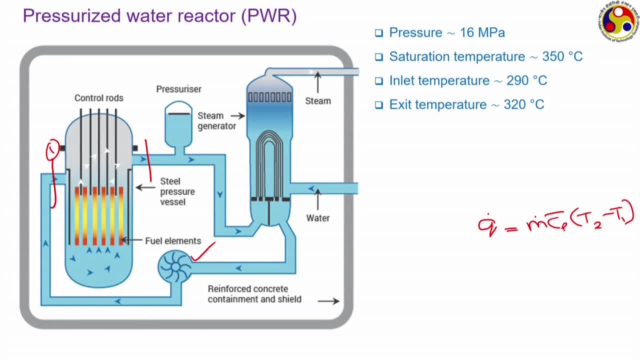 to keep. Now you will find that these temperature difference, that is, T 2 minus T 1, to some reasonable value of 25 to 30 degree Celsius And according with the outlet temperature of the coolant, which is expected to be the maximum temperature, that remains well below the corresponding. 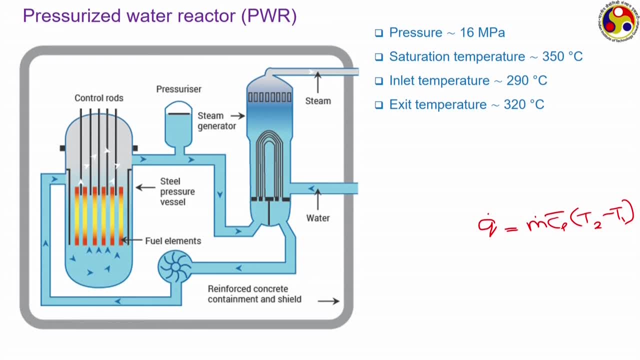 saturation temperature, thereby allowing single phase war pelosion throughout the loop, The secondary loop, where this water, which is coming from the reactor is transferring, it is heat that the pressure is something like 6 megapascal. only With respect to temperature change which is expected. the solution at the Twosome themselves. of T 2 is there In this. C 2 plus T 1 and T 1 would change JP pause's lower value toleras per minute, always for one second For the T 2 in C 2 plus T 1 up to 10 to 30 degree Celsius. 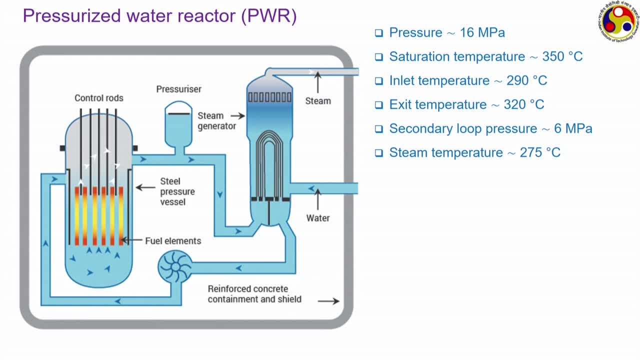 only And corresponding to that temperature. saturation temperature is around 275 degree Celsius. So the steam coming out through this particular point will be having a temperature around 275 degree Celsius and a pressure of 6 mega Pascal, Because the temperature of water coming here and entering the steam generator is of the level of 320 degree Celsius, a reasonable 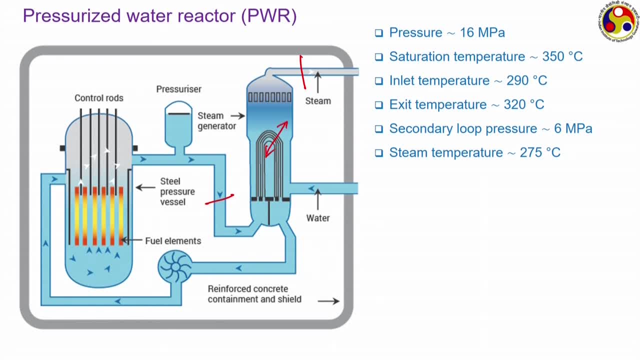 temperature difference can be obtained across the heat exchanging surfaces, here The pressure. then this steam is then taken to a Rankine cycle, which a conventional Rankine cycle, which may also contain reheating or superheating and even regeneration also, But that part is external, which is similar to any conventional coal based power stations. 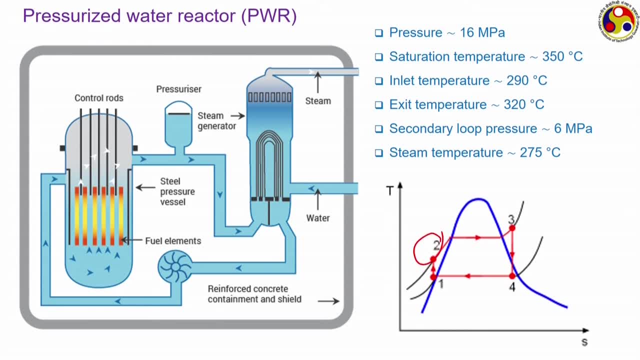 In nuclear power plant we only get as the operation between this 0.2 to 0.3, which is similar in conventional coal based power stations, the process that is done inside the boiler. But what is the process of the boiler? So? 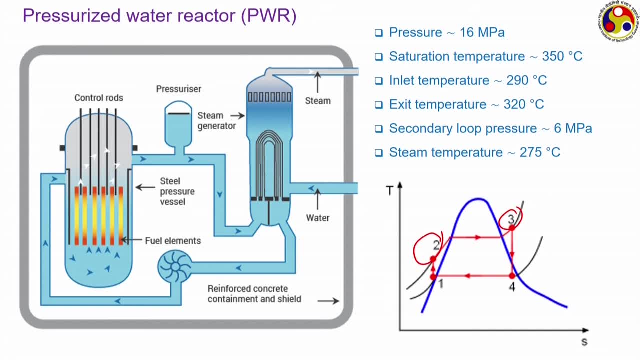 one difference with the coal based power stations to the PWRs is that the amount of energy raised is much higher compared to the energy. that is, energy released during fission is much higher compared to the energy released during coal combustion. But the question is, how can we ensure this system pressure of 16 mega Pascal Once we 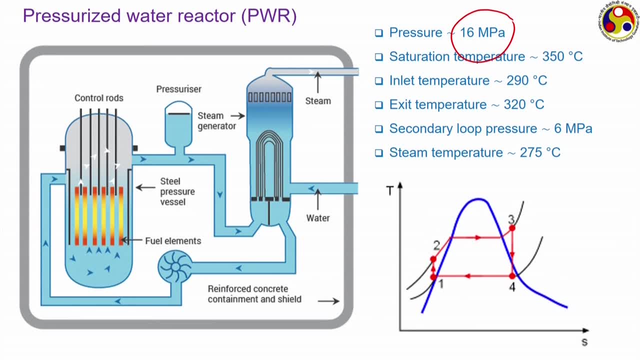 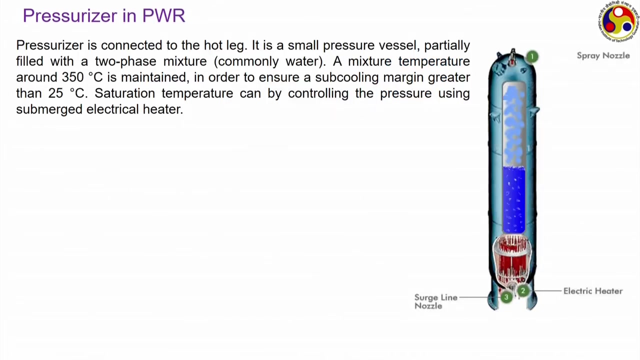 can ensure this high pressure. corresponding saturation temperature is already high and therefore by limiting the exit temperature temperature at this point, this T 2, we can easily easily heat upthe fluid or the steam here to any temperature of our choice. But the important part is we have to control the pressure that 16 m P a, and for that purpose 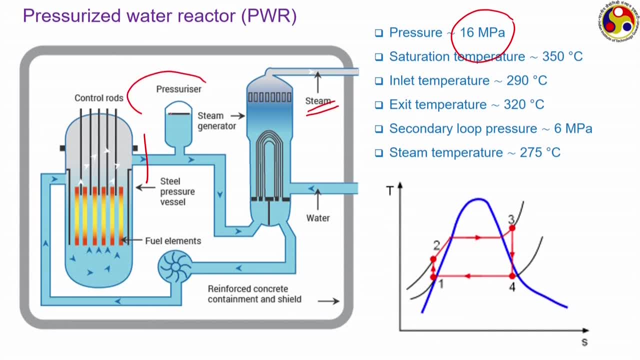 we have a pressuriser. this is the pressuriser that we have in a pressureised water reactor. a pressuriser is connected with a hot lake. conventionally, thisleg is called the cold lake and this one is called the hot lake. hasreacted with a hot lake, conventional this. 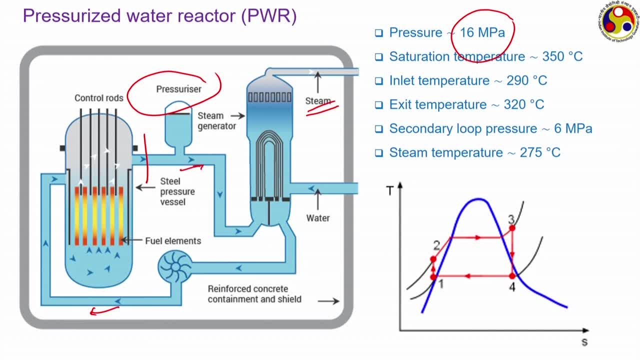 lake is called the cold lake and disone is called the hot lake, And this one calledy leg, because this hot leg carries energy of much higher level. The pressurizer is connected to the hot leg, through which it is able to come in contact. 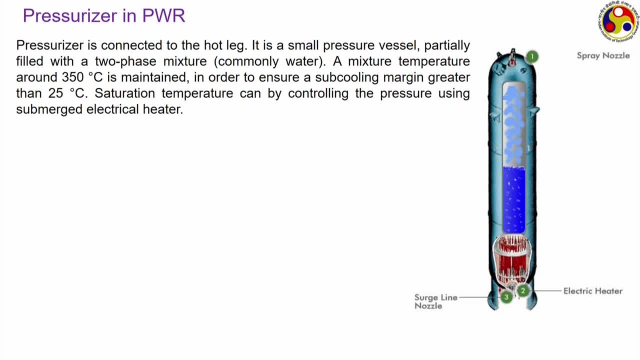 with the high temperature fluid. It is actually a very, very small pressure vessel. its volume is very small compared to the volume of the pressure original pressure vessel. but this small pressure vessel is partially filled with a two phase mixture which commonly is water itself. therefore, 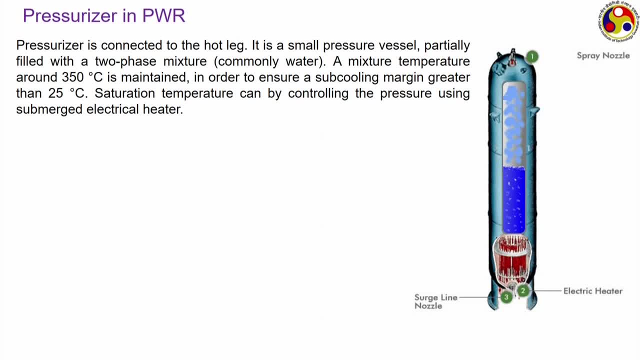 it can be said to be partially filled up with liquid water and water vapour mixture. We can maintain a coolant mixture temperature of 350 degree Celsius, which automatically can balance the pressure to the targeted pressure of around 16 mega Pascal, Because during the saturation state or whenever we are dealing with saturated mixture pressure. 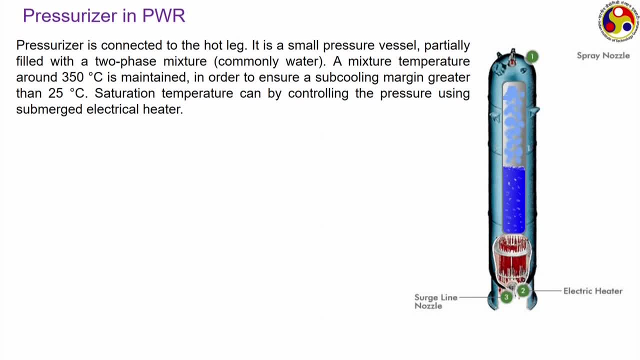 and temperature are not independent. rather, they are dependent on each other. once one of them is fixed, the other has to be fixed And therefore, by maintaining the temperature, By maintaining the certain temperature inside this, like 350 degree Celsius, we can maintain a pressure of 16- sorry 60. we can maintain a pressure of the order of this, 16 MPa inside. 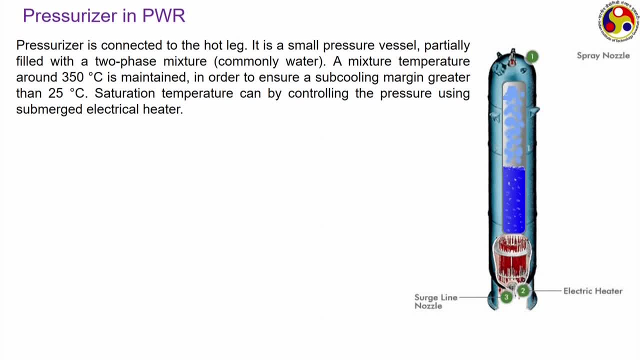 this reactor. The saturation temperature also can be controlled by varying a pressure and therefore we can maintain a fixed pressure and temperature inside the pressurizer. Because of this two phase nature of the fluid which is bound in this pressurizer, it is 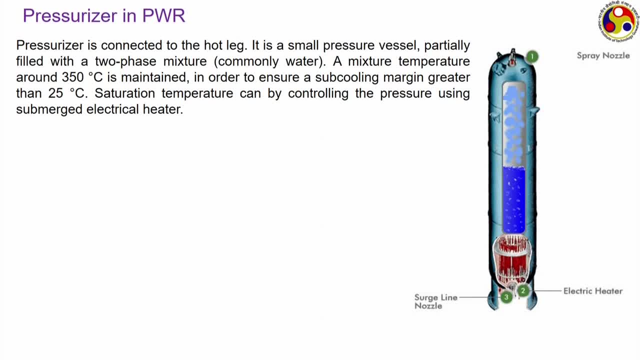 able to control the pressure inside and also it can absorb any kind of pressure upsurge or downsurge which may appear during any operation. Now, whenever there is a pressure upsurge, that is, there is a very small increase in the pressure inside the actual pressure vessel, then that will cause a rise in the water level inside. 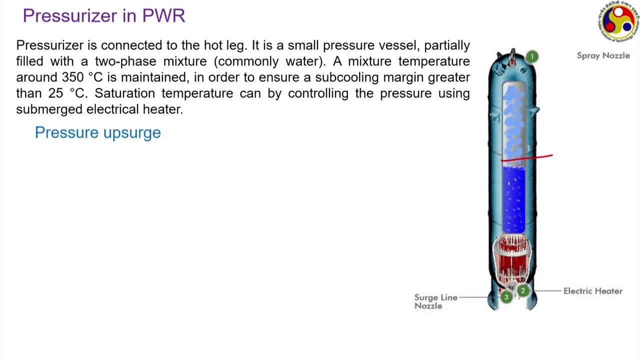 this pressurizer water, the liquid part, that being incompressible in nature. so there will not be too much change in the volume. rather, the water level inside this will rise a bit And once the water level is rising, that will result in a reduction in the volume available. 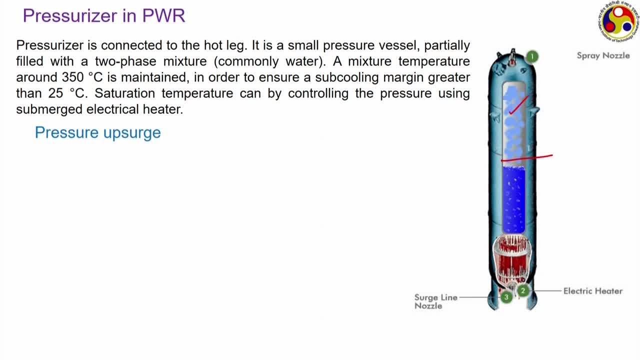 to the vapor phase which is here. So the vapor phase will get compressed a bit and whenever the vapor phase gets compressed we have one spray nozzle mounted here. this spray nozzle gets activated and this spray nozzle some cold liquid water on the vapour. somewhere here the spray nozzle will put the spray. 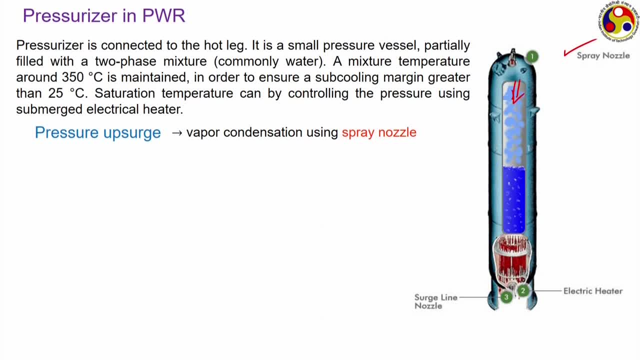 somewhere here, thereby condensing some amount of vapour. and once the vapour condenses, so the pressure of this vapour part reduces accordingly. It can- it can able to capture or retain a new equilibrium corresponding to this new position of this free surface. 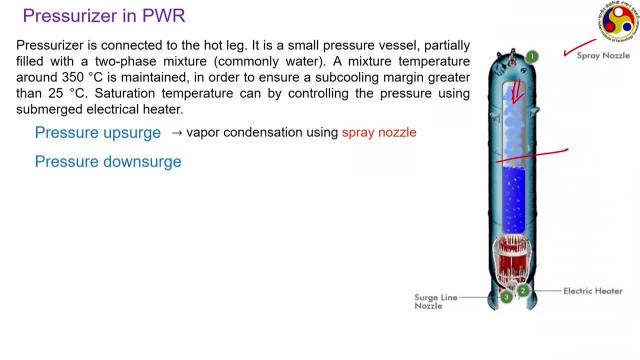 Similarly, whenever there is a pressure down surge, if the pressure inside the container main reactor vessel reduces, then that will also draw a little bit of liquid out of this pressuriser and so the pressure. there is now higher volume available for the vapour which 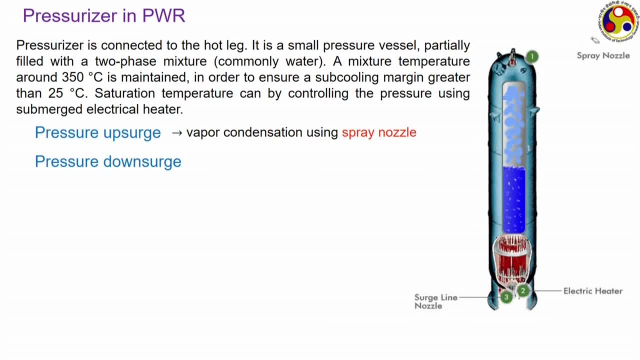 is present higher volume of vapour available which in this portion. So this vapour will try to expand. but as the pressure has fallen, But both liquid and vapour part remains, are the saturation temperature corresponding to the initial higher pressure. So some liquid from this free surface will try to evaporate. 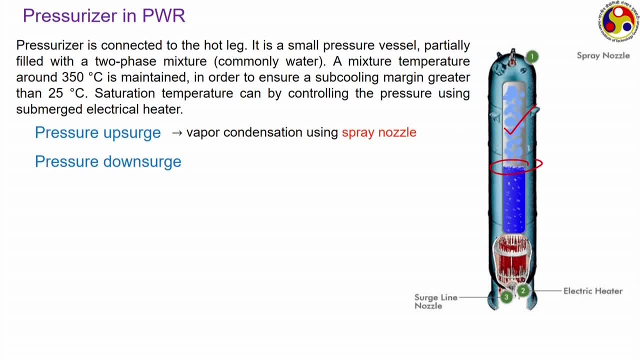 and occupy that portion, thereby gaining a equality. equality or equilibrium in terms of pressure. I think I told something wrong. I would like to correct this once more. Whenever there is a pressure down surge, there will be a reduction in the free surface level. 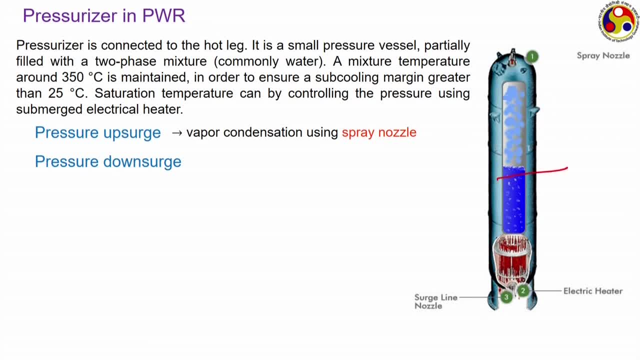 So the free surface- The free surface, say- has come down here, So now larger volume is available for the vapour phase and hence the pressure on the liquid surface. that also reduces, and because of that some liquid from this portion, as both liquid and vapour part, are already in the saturation. 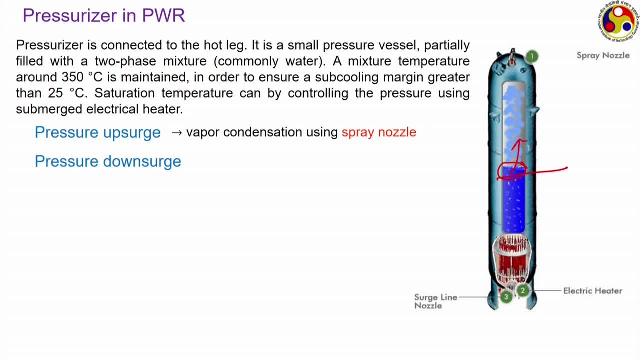 temperature, So that will evaporate or that will flash into vapour and occupy this portions, thereby contributing more molecules to the vapour part. That increases the pressure in the vapour part and hence is able to attain the equilibrium, Or the entire system can go back to its original position If the flushing itself is not sufficient. 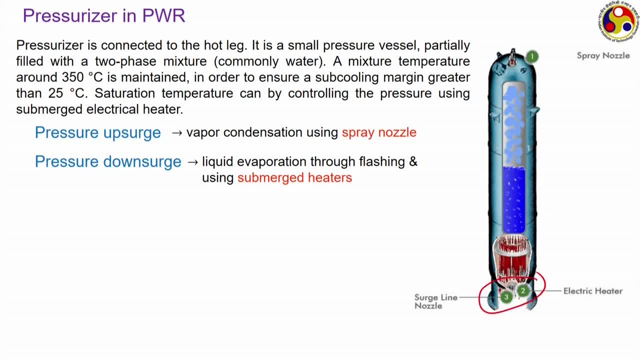 then we may have submerged electrical heater here. This electrical heaters also can get activated and heat of the liquid, thereby leading to some further evaporation of the droplets and getting the pressure level back to the original one. So pressurizer serves several purposes, and the first one is the pressure control. Like I have mentioned earlier, we 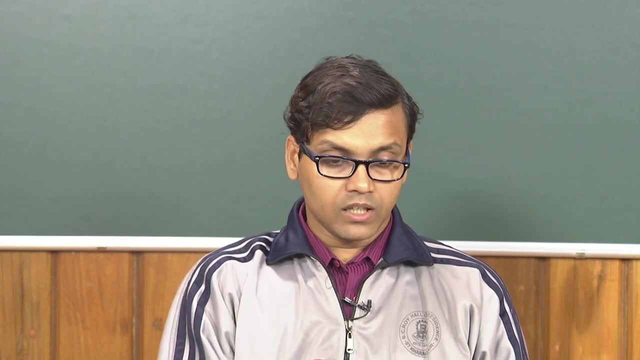 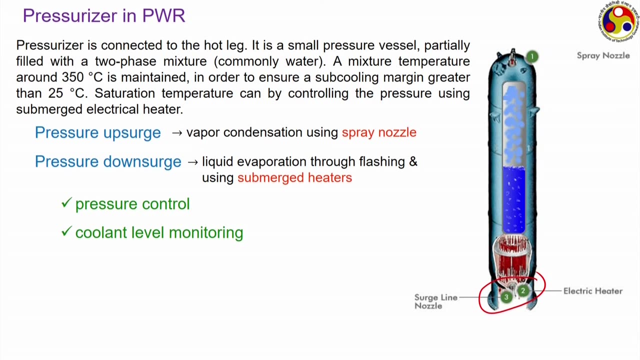 have mentioned, both pressure upsurge and downsize can be maintained. Another function done by the pressurizer is the coolant level monitoring. Generally, the pressurizer is mounted at the top of the pressure vessel, which is likely to be the highest location. 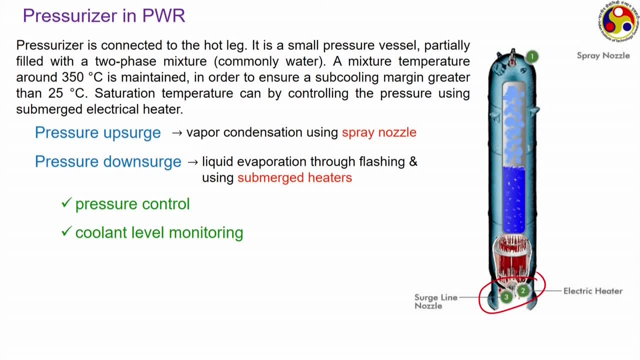 of the plant And hence, if the pressurizer is having sufficient amount of liquid, then all components which are placed at a lower elevation has to must have the must have some sufficient amount of liquid present. Therefore they are just by observing the coolant level. 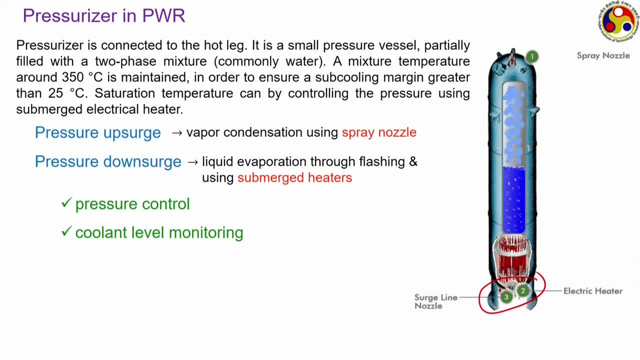 inside the pressurizer we can know the pressure of, or I should say we can ensure that what there is sufficient water throughout the reactor system. And the third is overpressure protection. Somewhere here on the top of the pressurizer there will be a safety valve If there is a certain overpressure in the system, which 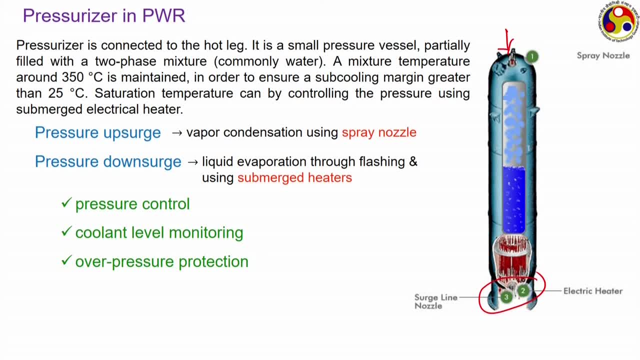 the pressurizer is also not able to control, So there is a safety valve. So if there is a certain overpressure in the system which the pressurizer is also not able to control, it will take care of it. to this overpressure protection valve opens, allowing some steam. 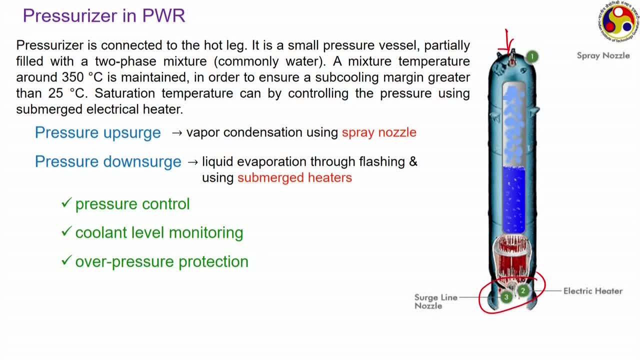 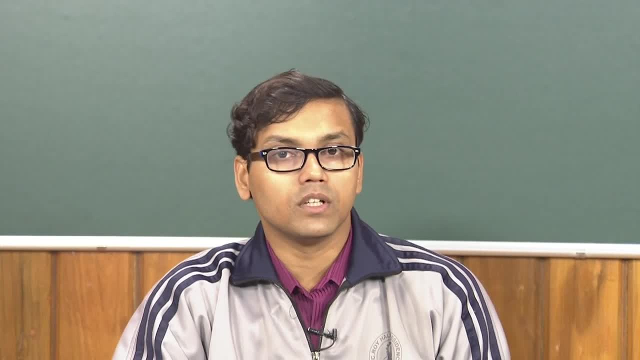 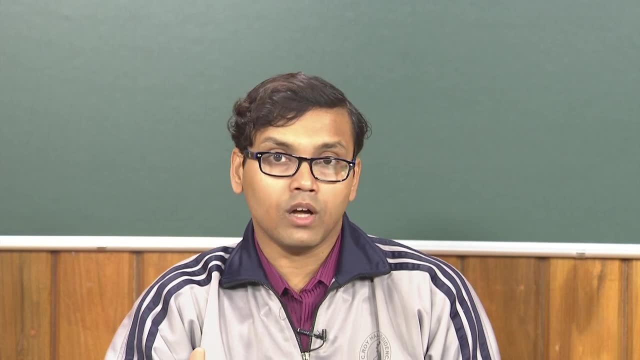 to escape. You can think this one- or you can- to be analogous to the safety valve that we can have in a pressure cooker. Whenever the pressure inside is high, then the safety valve opens, allowing some steam to escape and thereby gains the equilibrium back. However, if the control valve is not sufficient or the safety valve, 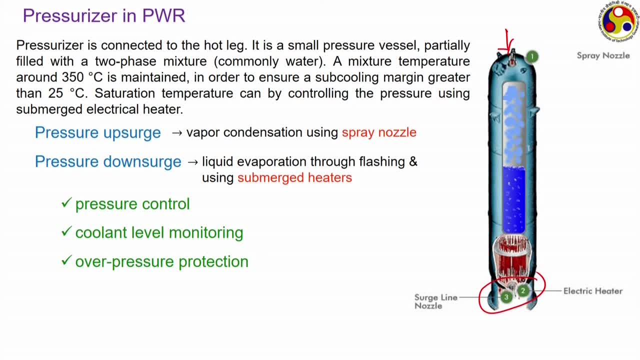 is not sufficient. So there will be another emergency protection valve on the lid of the pressure cooker, So in case of emergency that opens, allowing some further release of vapor phase. This overpressure protection is also somewhat similar kind, Whenever there is some excess pressure, which 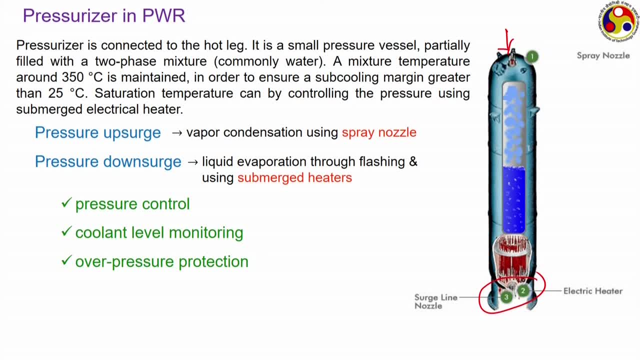 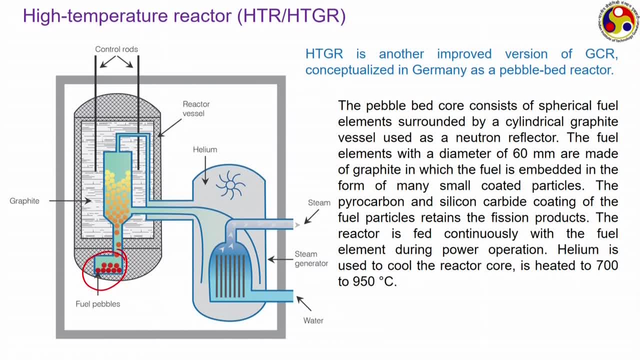 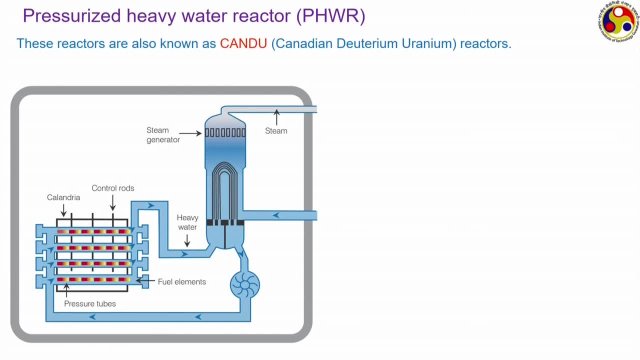 this kind of reactors are also called CANDU reactors because they are originated from Canada and the term Canadian deuterium uranium combines to this pressurized heavy water reactor. Here the most striking feature is the pressure tube type design. We have a large vessel here. 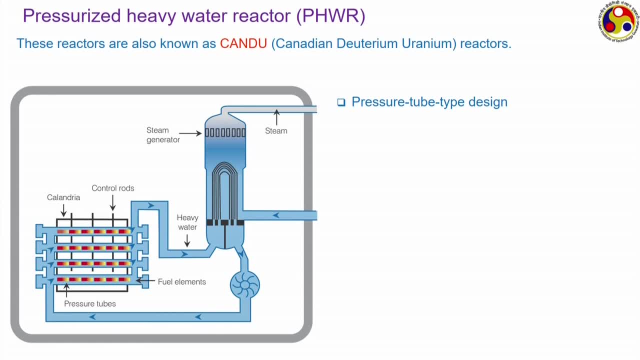 which is which is called calendria. inside the calendria we have heavy water stored And then the several pressure tubes are immersed into this calendria, which the tubes which are containing the fuel elements, The coolant that is allowed to pass over this pressure tubes, thereby absorbing the energy. So the D2O is stored in the calendria and several 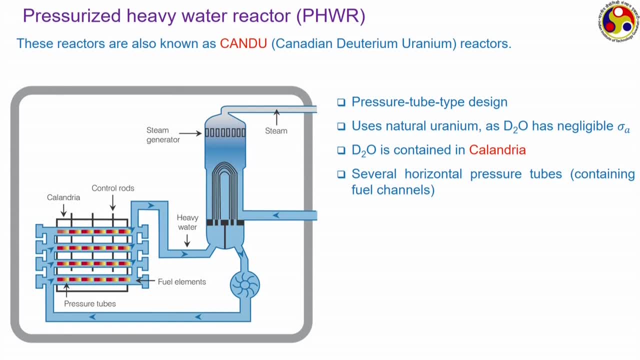 horizontal pressure tubes containing the fuel channels. they are also immersed into that Ah. They also quite similar to this RBMK group of reactors. they can also be refueled at full power, allowing very efficient use of uranium, And that is why the CANDU group of reactors, or the PHWR, has become very popular, particularly. 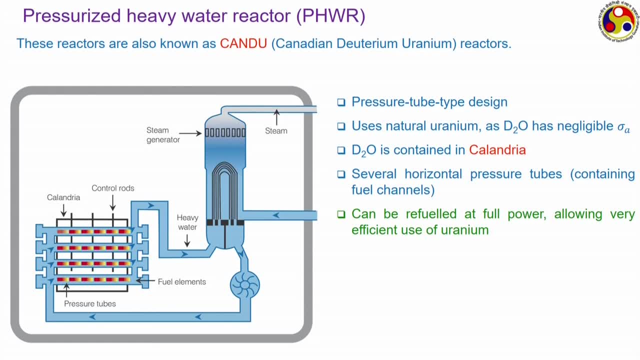 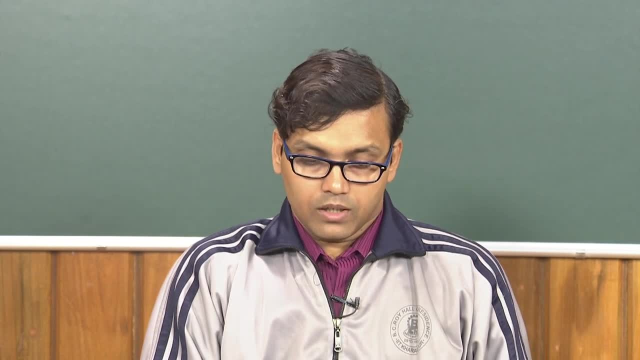 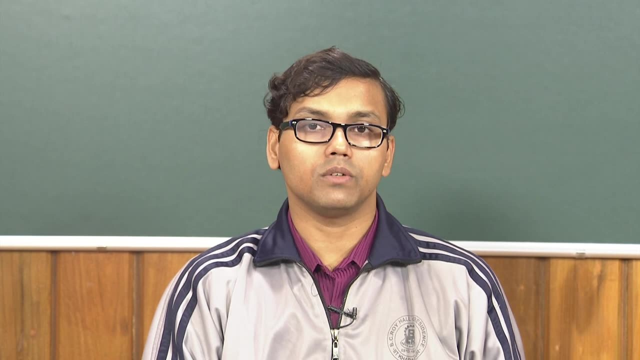 in India. Apart from the initial PWRs, almost all Indian nuclear power stations employs PHWR kind of nuclear reactor. As we are using heavy water, it does not have any absorption cross section, or this absorption cross section is negligible. That is why we can use natural uranium, and hence the fuel cost is significantly reduced. 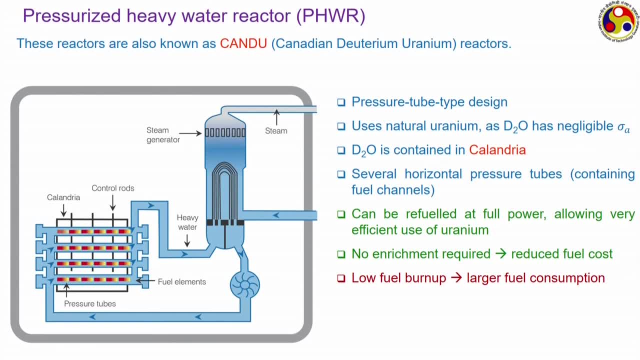 But one problem is that the burn-off is low and therefore fuel consumption rate also will be much larger. And another big issue: heavy water itself is very, very expensive, and so whatever gain in terms of cost we get by using natural uranium, whether that is competitive or competitive- 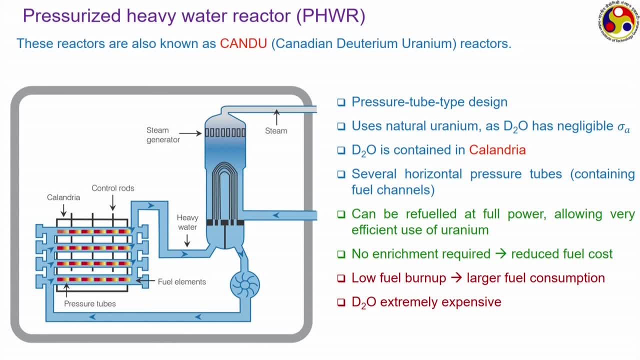 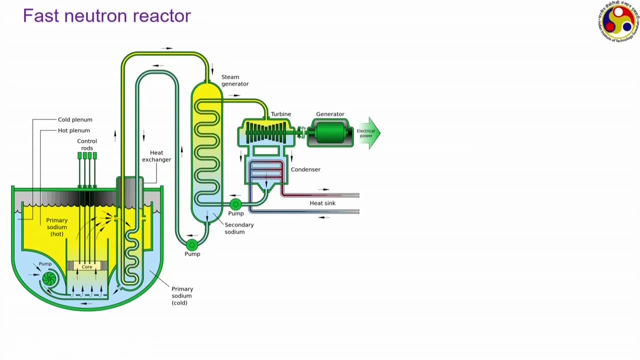 compensated, or whether that is compensated or not. that we have to be careful of. And then we come to the last one is category, which is fast neutron reactor, which is, truly speaking, is not a thermal reactor, rather it employs fast neutron, still for the purpose of completeness. I am mentioning this: 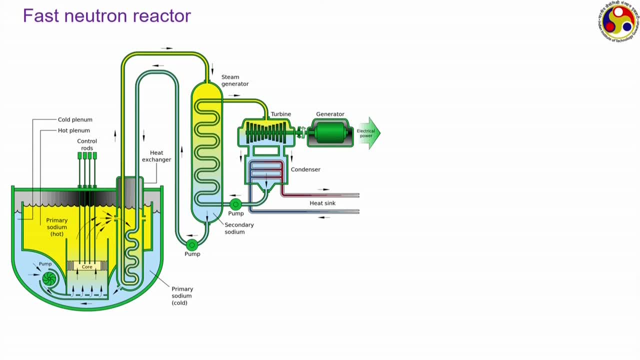 Here there are no moderators, because we are trying to use the fast neutrons And as there are no moderators present, so there will be significant excess of neutrons. Moderators- Moderators can itself also eat up some amount of neutrons, and that portion is not present. 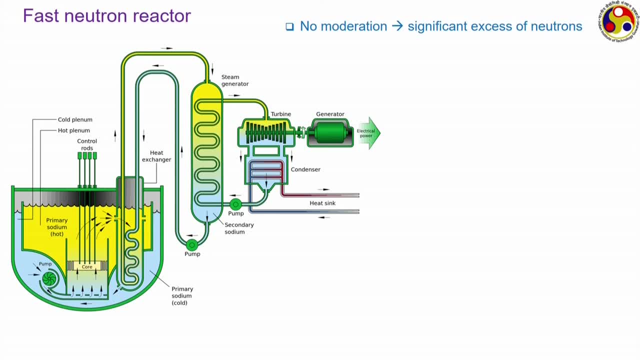 and also as the moderators are not going through- sorry. the neutrons are not going through any kind of scattering or slowing down process, So they are not likely to enter the resonance absorption zone. So the there will be no resonance absorption as well. 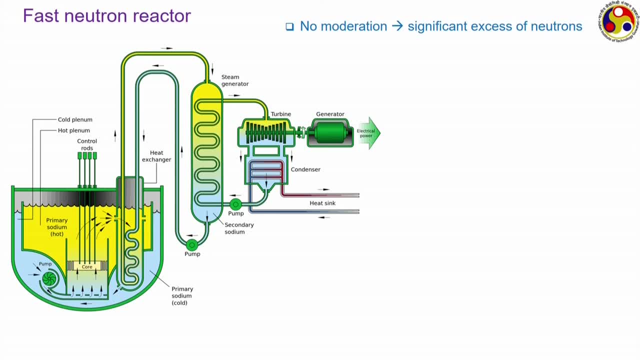 That is why fast neutron reactors have significant excess in terms of neutrons. They also requires, So a highly enriched fuel of the range of 10 percent or even more, but they because of such high neutron excess. we generally need to have a very compact reactor core. 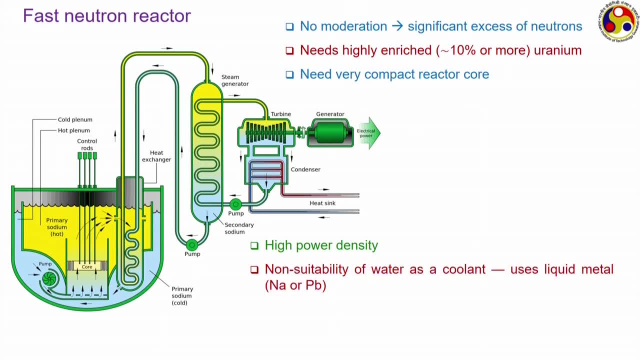 And we resulting in high power density. so but one big problem for them: water is not suitable as a coolant because of two reasons. common water has a little bit of capture, cross sections, So it can reduce the neutron density, And also the because of such large number of neutron presence and also the being the. 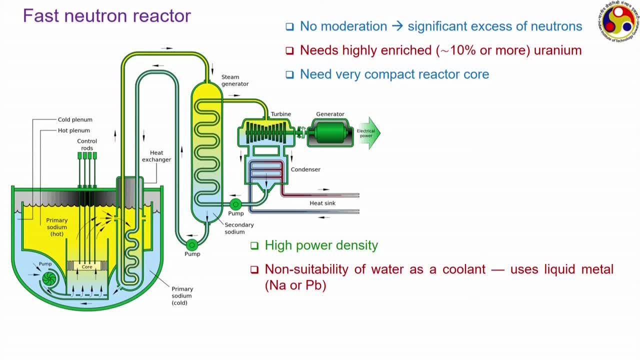 fast neutron lifetime being quite small, or prompt neutron lifetimes being quite small, The rate of power production from this PHWR is very high, and that is why water is not capable of carrying that amount of energy And we have to use some kind of highly conductive fuel that needs to be used, something like 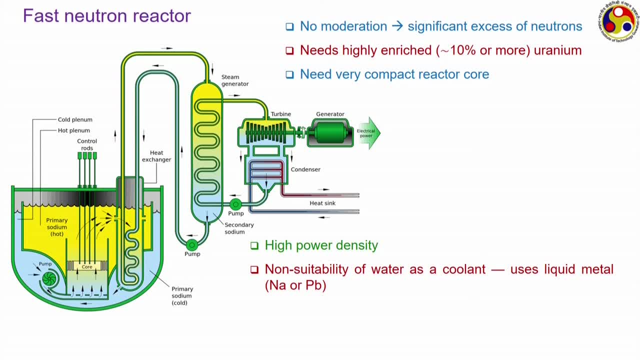 liquid metal such as sodium or potassium. So if you follow the diagram here, this is a primary sodium which is flowing to the core and then that is getting pumped where- this into the core, So it passes to the fuels and comes out as high temperature sodium. 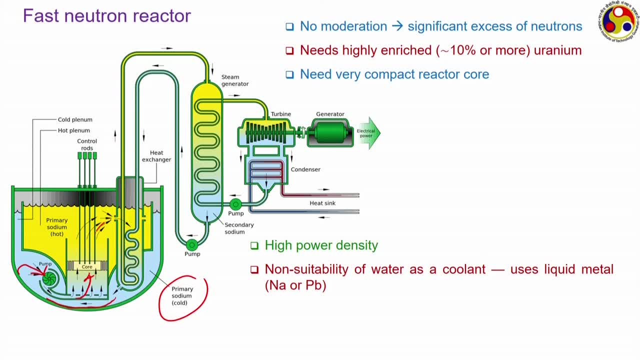 That sodium is passing through the core, So it passes through the fuels and comes out as high temperature sodium passing through or passing over a heat exchanger and the other side of the heat exchanger. we also have again liquid metal And this- this is the secondary loop which is taking this. 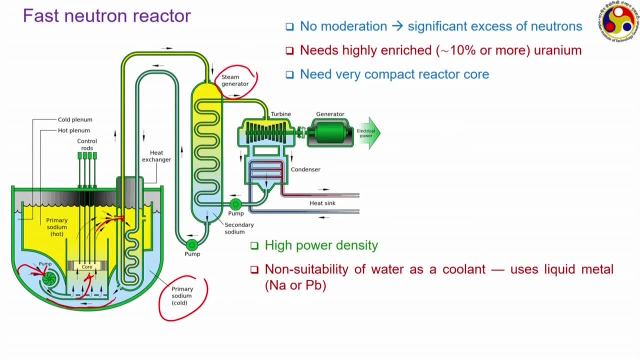 energy towards outside, to a steam generator where this energy from the secondary loop is being transferred to water. So we are using sodium in both primary as well as in the secondary reactor or secondary loop. So this secondary sodium loop, which can help us avoiding radioactive effect, also complicates the design and put some additional burden. 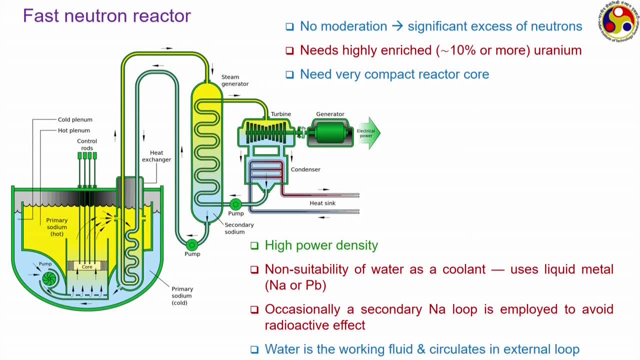 on fabrication point of view, The in the outside loop we use water only, which gets the energy from this second sodium loop and then in a conventional Rankine power cycle it can produce the power. Fast neutron reactors essentially employs a technique called breeding By virtue of 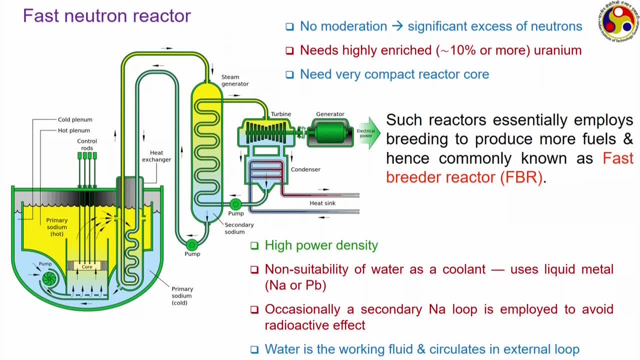 breeding. it can convert fertile material to fissile materials, and thereby it can produce some more fuels. That is why fast neutron reactors are also conventionally called fast breeder reactor, FBR, which is the topic of our discussion in module 8.. So it takes me to the end of this particular lecture. Here we have discussed about some 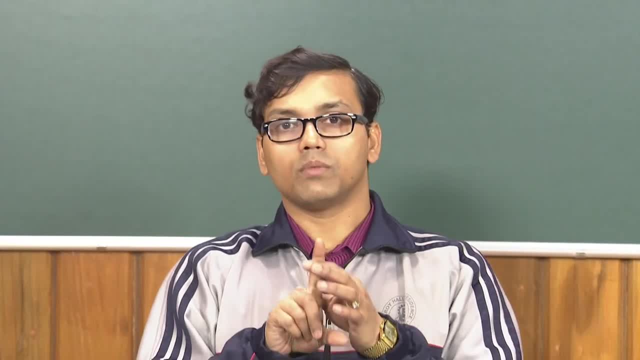 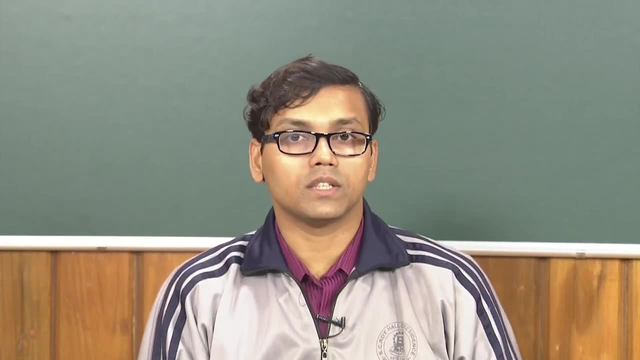 of the conventional reactors. So we have discussed about the conventional reactors. We have talked about conventional nuclear reactors like the pressurized water reactor, boiling water reactor, advanced gas cooled reactor, pressurized heavy water reactor and also the fast neutron reactor. And as a variation of this advanced gas cooled reactor, we have